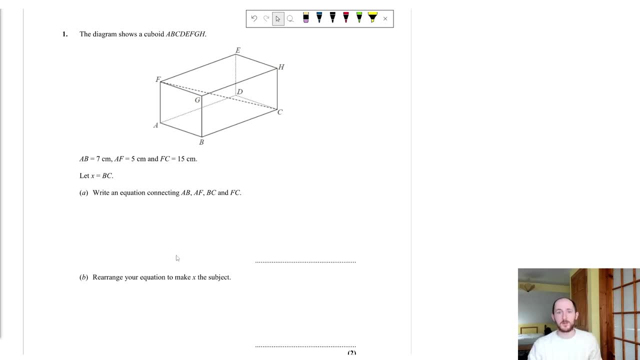 this one has been written in a way where it's slightly more difficult to find out what you need to do. So again, remember the grade 9 questions. they are the 10% unseen marks where they put you in a situation you haven't been in before. So, for example, with this one, you know you. 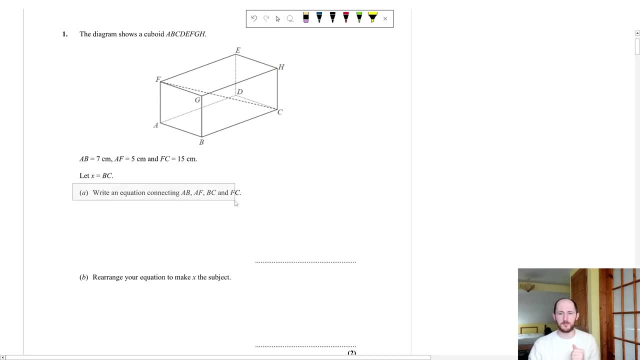 might recognize it as 3D, Pythagoras or trig, but write an equation connecting A, B, A, F, B, C and F C. That's kind of weird, right? That's different. They've written it in a slightly different way. 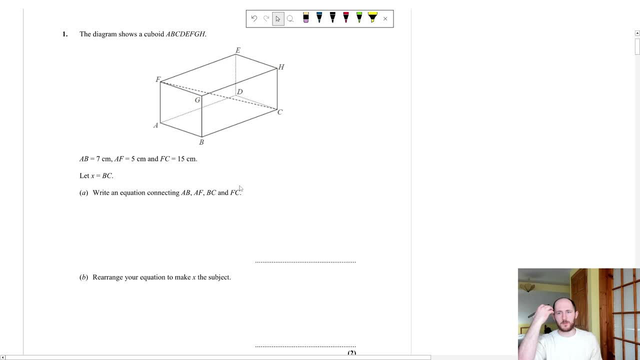 So I thought again: I've collected these questions, I'm going to go through them, talk through my thought processes and we'll see how far we get. So, without further ado, let's jump into question one. So we have a cuboid, Wonderful, And I like to label the sides myself. So write in the information. So 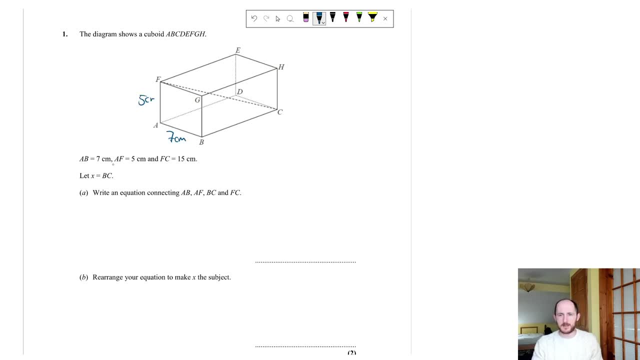 A- B is 7 centimeters, A- F is 5. Centimeters And F- C is 15.. That's kind of a hard one to write, And if you look ahead at part B, actually never mind, I don't know what I was talking about- It says: let X equals B- C. 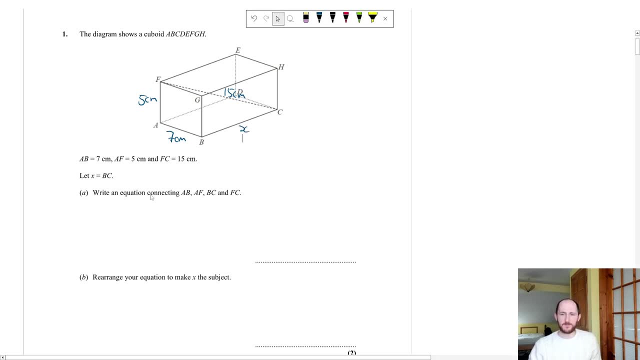 So essentially in the first question we're writing the equation connecting A, B, A, F, B, C and F, C. So I would probably write those as numbers, but let's leave them as letters for now. And they've given us a hint by saying: let X equals B, C. 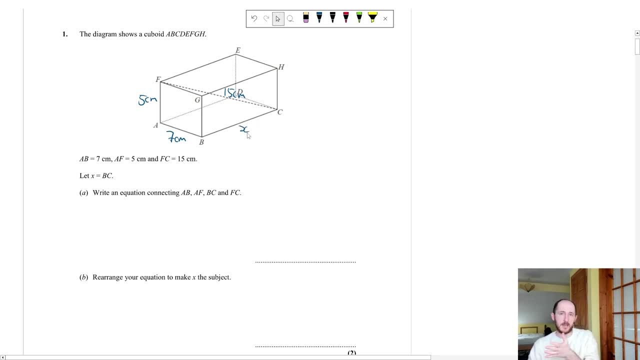 Because all we're going to do is try and find an equation in terms of X as in 4X. So how do you do 3D trig? Well, of course, you're going to break it up into different triangles. Now, the reason why I said 3D Pythagoras first is because if they don't give you angles and you don't- 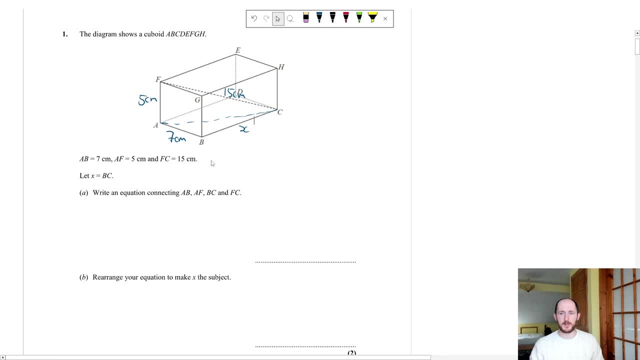 need to work out an angle, then it's going to be Pythagoras, not trig, So that triangle here looks like this: F, A, C, AC- I don't know AF is well, they want me to leave it in terms of AF, BC and FC. So sure, whatever. 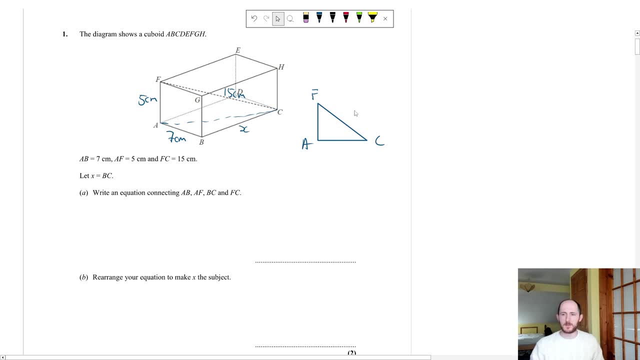 right, that's fine if they want me to do that. And the reason why I want it is if I look at the side X again, if think of Pythagoras, that makes up a triangle that looks like this. But we have A, C and B, right. If I look- look at this cuboid from top down, I have ABC, that's a. 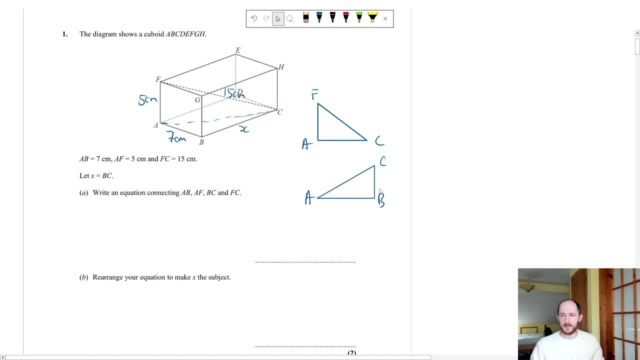 triangle. I want to work outside BC, this side- but in order to do that, I need to know both of these other sides, and I know one of them, but I don't know AC, The other way. the other reason why I know that I need to do it is because I need to connect all four sides. So what I'm going to do is because 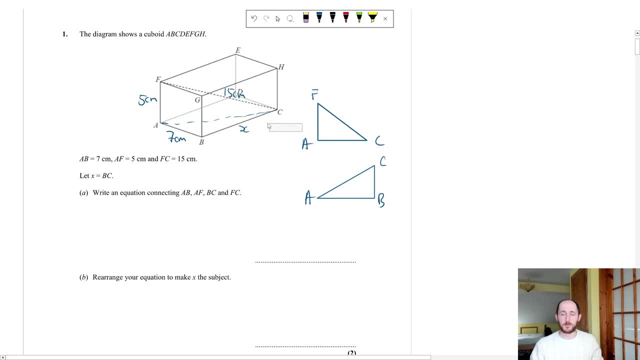 AC is shared between the two expressions. I'm going to write it out. So what would trig look like in this case? Well, it would be: FC squared is equal to AF squared plus AC squared. So I've got AF, FC and AC. but if you notice, AC is not in this expression, it's AB. 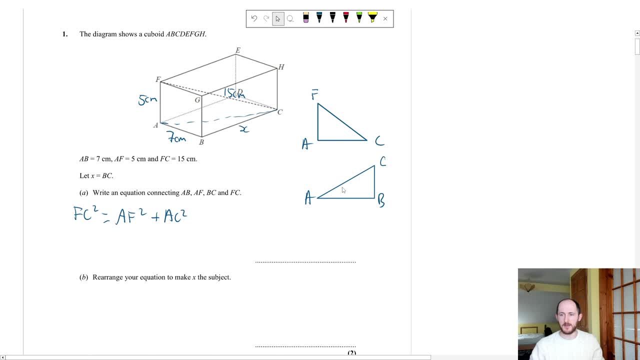 and BC. So I'm going to use AC from here, which would be: AC squared equals AB squared plus BC squared, and I'm going to sub that into this expression. So we have FC squared equals AF squared plus AB squared, And, as you can see, we have FC- FC, We have AF- AF, We have AB- AB, We have BC- BC. So that's how I'd approach that question. Again, in a normal situation, though, just say: hey, work out the length BC, which is what they're going to do towards the end. but it's just a weird way of them putting the first question, because they want to see if you can form equations. Part B: rearrange your equation to make X the subject. Don't forget let X equals BC. so I could. 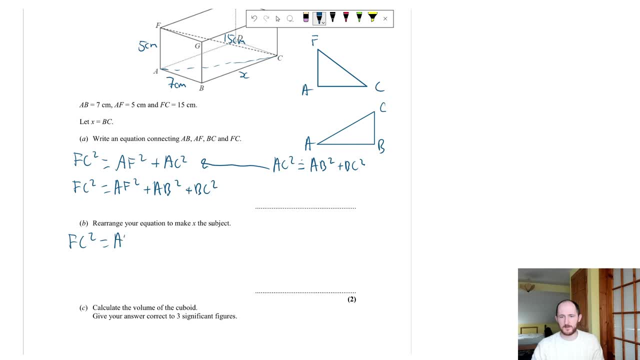 write that equation as: FC squared equals AF squared, plus AB squared plus X squared. So if I'm rearranging it to make X the subject, it will be: X equals FC squared minus AF squared- God, I don't know what I'm trying to write there- Minus AB squared. and then, don't forget, it's rearranging to make X the subject, not X squared, so the whole thing is going to be square rooted. 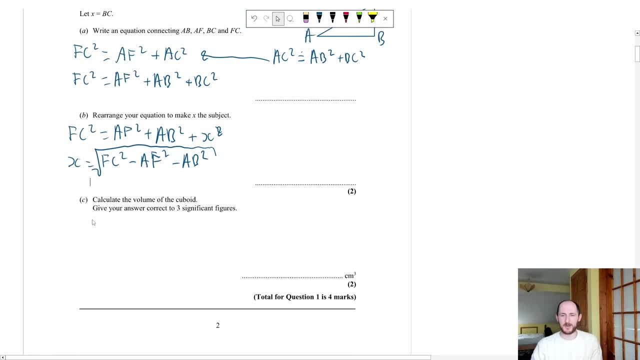 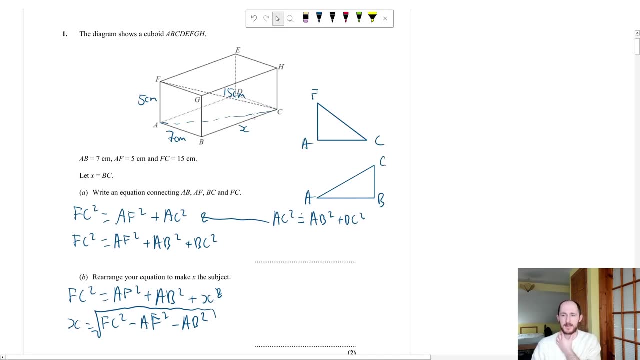 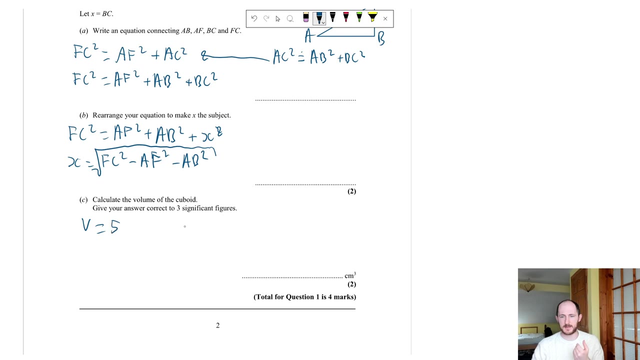 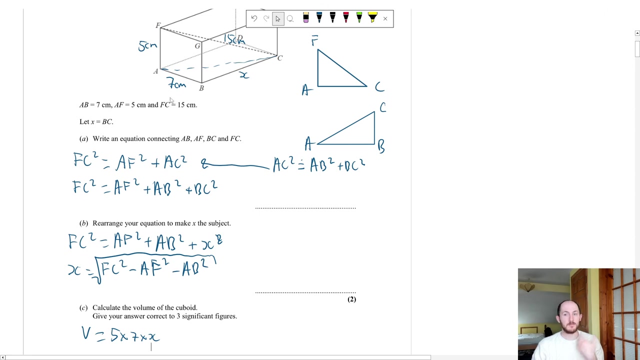 Lovely, Two marks only, which is a bit funny. but calculate the volume of the cuboid, Remember to do the volume of any kind of prism, you need the front area times by its length. In this case it would be 5 times 7 for the area times by X. So it's just 5 times 7 times X. I need to work out what X is, so I'm going to substitute into this formula that I worked out, hence why they did it in the first place. So I'm going to use my calculator, of course. so I'm going to use my calculator, of course. 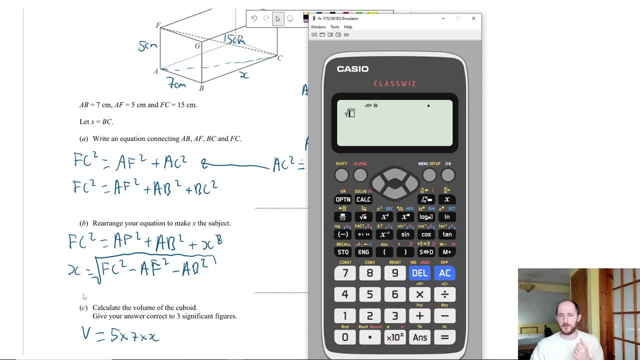 bring that out: Square root, fc squared. so fc was 15, squared af, af was 5.. ab was 7.. We get square root of 151.. Not really that helpful, but we'll leave it as is for now. 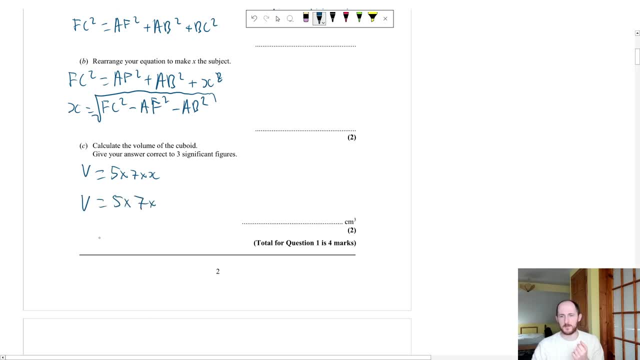 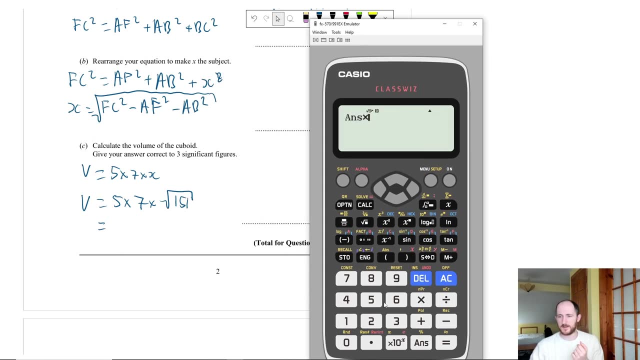 So the volume is just equal to 5 times 7, times the square root of 151.. And we need to give this to three significant figures. So times by 5 times by 7 gives me 430.. That is 3sf, so that's nice. 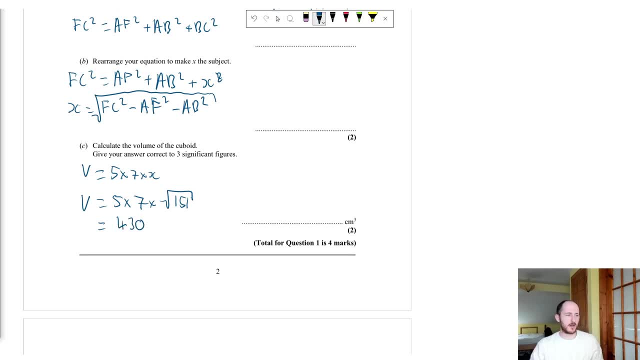 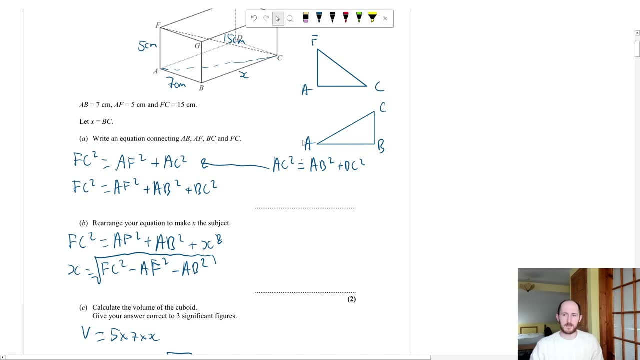 And that's it for the first question. So again, under normal circumstances the question wouldn't be too bad, but definitely this first part would throw quite a few people through a loop. But again, it doesn't matter if we're using letters or using numbers, it's the same process. 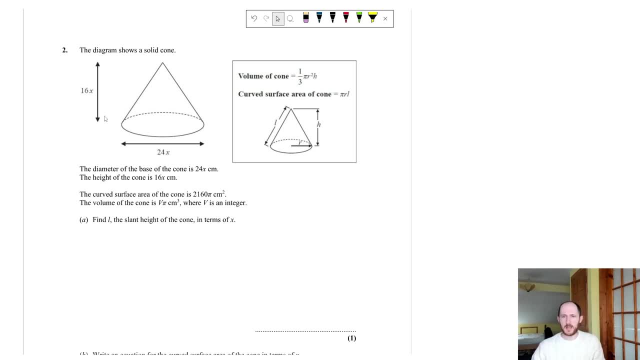 So here we have a solid cone and it gives us the diameter and the vertical height of the cone in terms of x, It gives us the curved surface area in terms of pi and the volume, And it takes you through kind of the steps on how to work out the value of v, so the actual value of 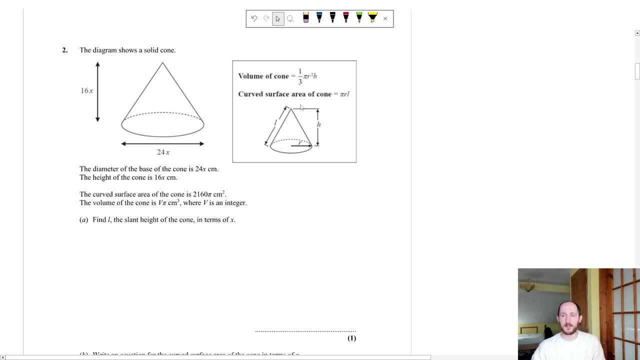 the volume, And the first step is to find the slant height of the cone in terms of x. Now some people might be tempted to just sub in for the curved surface area of the cone and rearrange, But we need to keep this in mind. If I do that and I work out what l is from this equation, 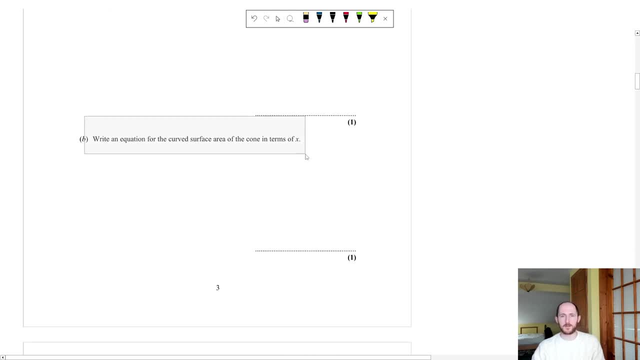 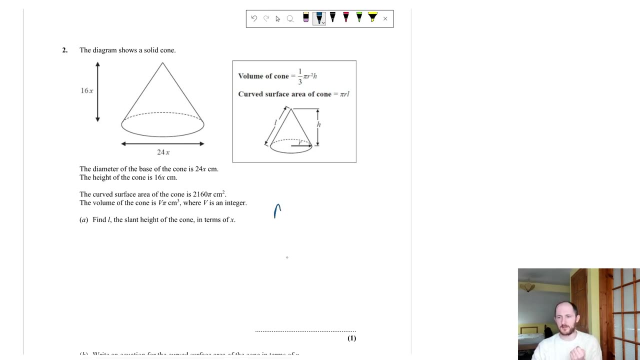 I will not then be able to sub it in for the curved surface area because it will all cancel out, Right? So let's say I had an equation like this: where it's the curved surface area, so the area is equal to pi r l If I rearrange it for l, so then I get l is equal to a over pi r, and then I sub it. 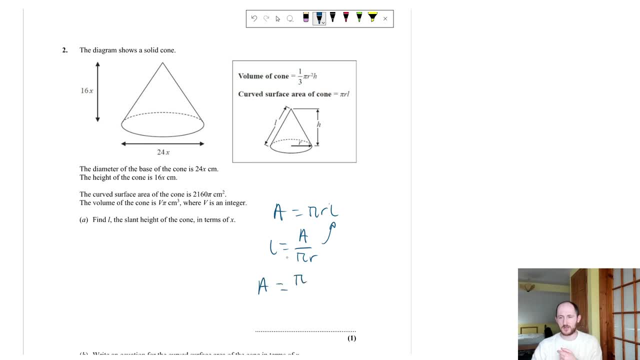 back into here. it's not going to work because it's going to give me an answer that's really nonsensical. So it's going to say a is equal to a And it's like: well duh. So if you try and sub in for the curved surface area of 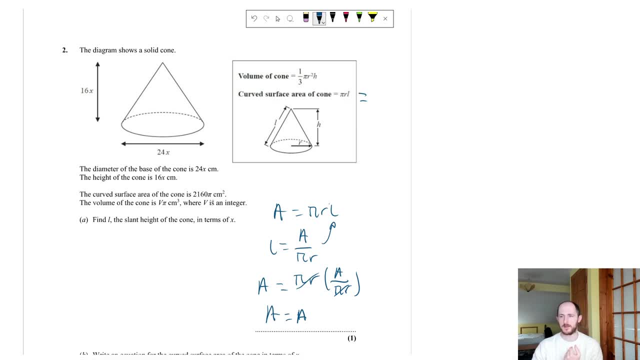 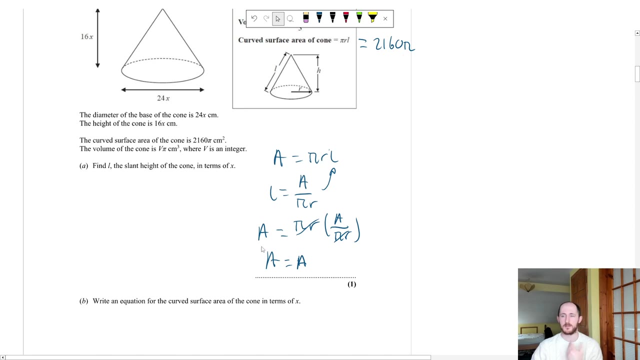 the cone equals 2160 pi and you try and rearrange this for x or for l. sorry, when you do part b, you'll get an answer which will just say something like: x is equal to x, which is not. 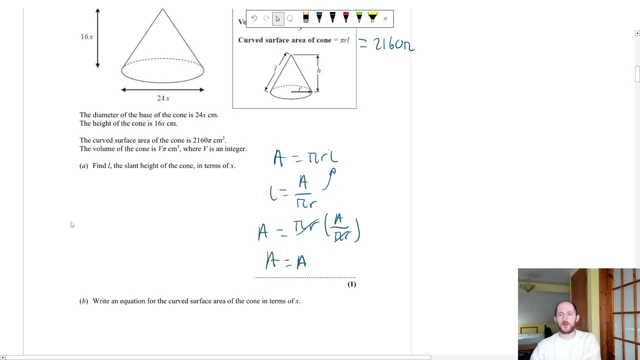 useful. The reason for this is, mathematically speaking, rearrange an equation and then sub into that same equation. It won't work In the same way that when you do simultaneous equations. when you rearrange one of them and you substitute it in, you can't. 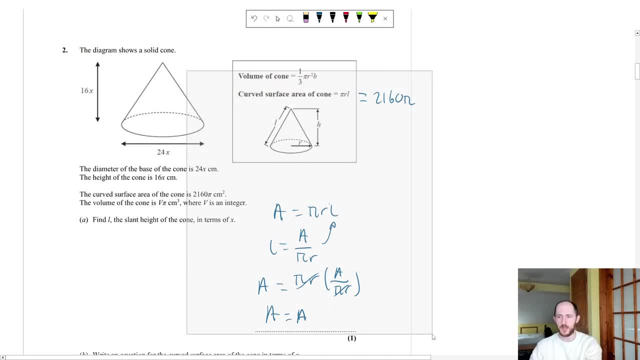 sub it into the same equation, Otherwise it gives you something nonsensical. So we need to find another way of finding x, an expression for x in terms of L. I hope that's a satisfactory response, But if you don't believe me, do what I just said and see what happens. 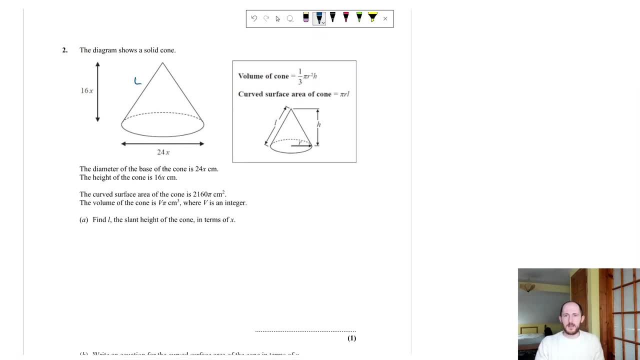 So L is the slanted height. If I move this 16x over, so it's the height of the cone. I mean I guess it wouldn't technically be all the way down there- The radius would then be 12x And if you look it makes a right-angled triangle. 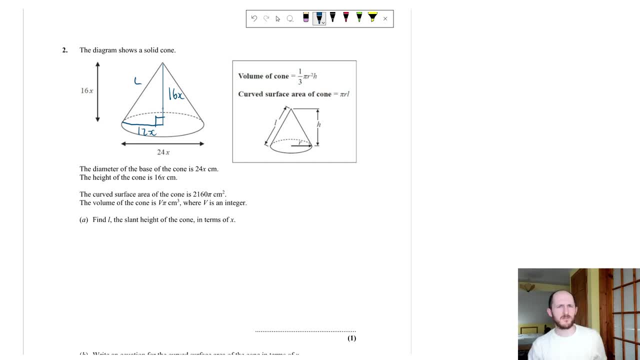 So I'm going to use Pythagoras to work out a value, not a value, an expression for L. So L is going to equal the square root of 12x squared Plus 16x squared. So let's quickly do these together. What I could do to make my life a. 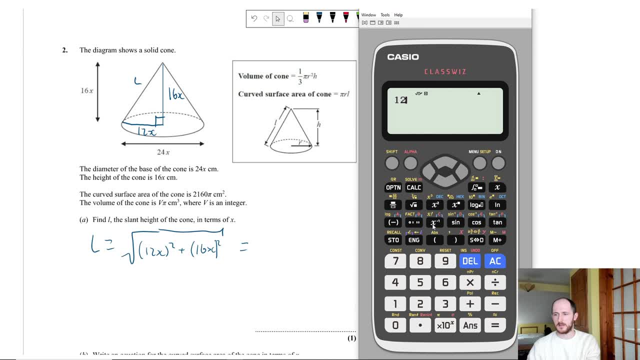 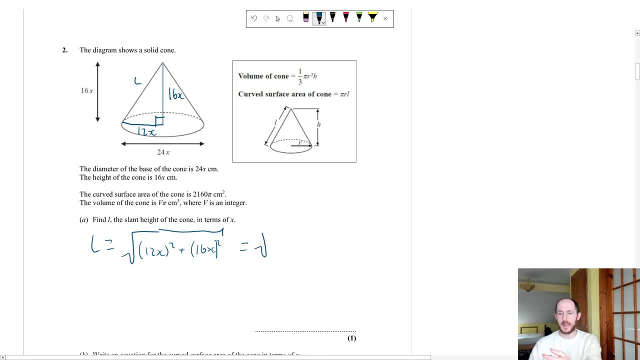 bit easier is actually do 12 squared plus 16 squared, Because I know that the x- x are both going to be x squared, So that's 400 squared, 400x squared, And then when I square roots we get 20x, So L is equal to 20x. That is the intended solution, okay. 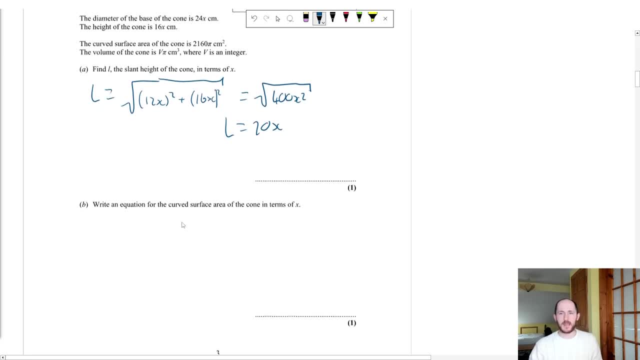 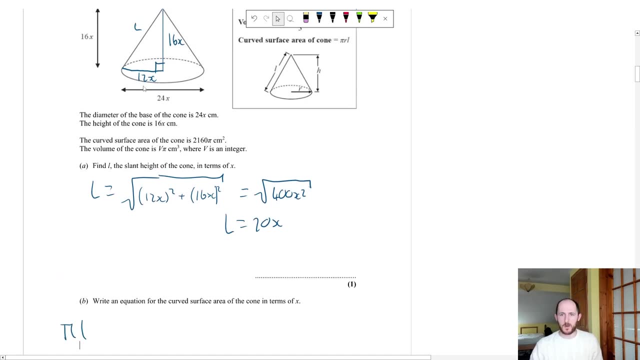 For part B, finding an equation for the curved surface area in terms of x. Now we use that. So we have pi R, L. Well, pi is just, pi, R is 12x And L. well, we don't want two unknowns. 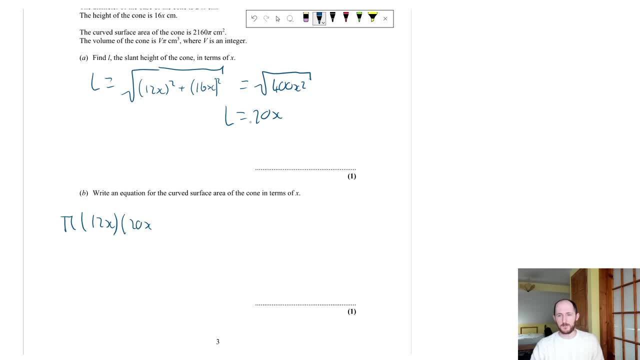 So we're going to just sub in 20x, for L equals 2160 pi, So we can cancel out both pi's. 12 times 20 would be 240 pi. No, it would be more than that, wouldn't it? No, it wouldn't, It would be 240x squared. 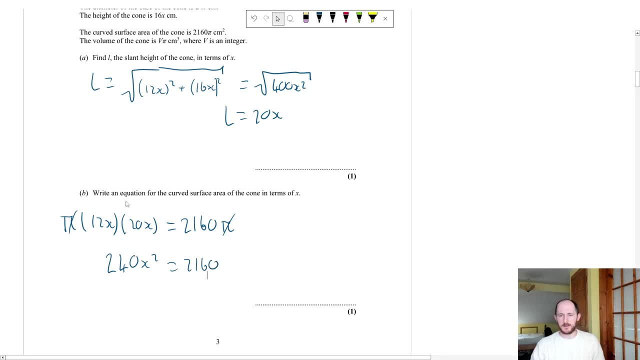 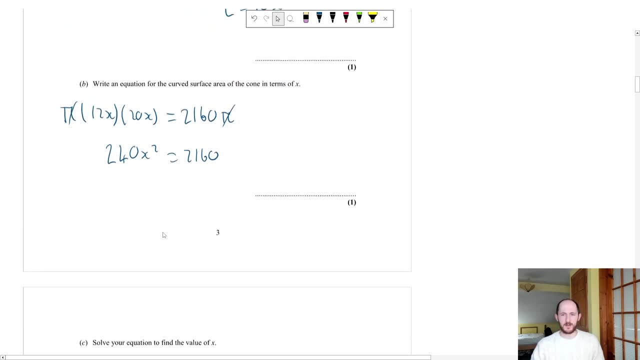 equals 2160.. I can then. I mean honestly this should be fine, But if not, we could rearrange for x. It does say part C: solve your equation to find x. So this should be perfectly fine, Or maybe even this first step. Again, don't forget these questions that I 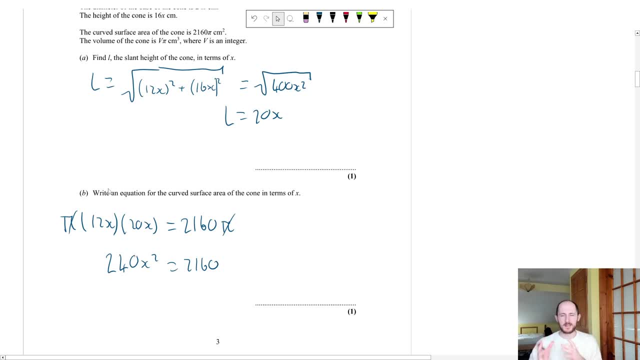 found. they are harder, But they're also written in a slightly different way to the normal exam. So this is going to be predicted for grade nine, right? So how they could potentially mess you about, so to speak. Solve to find x. Well, that's nice and easy. x squared is. 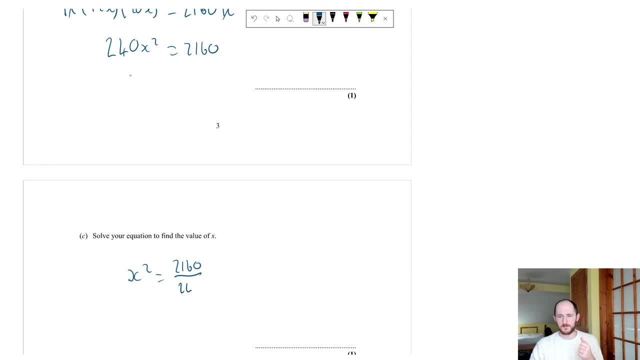 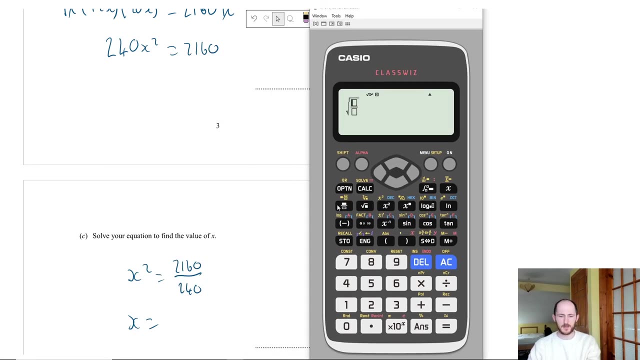 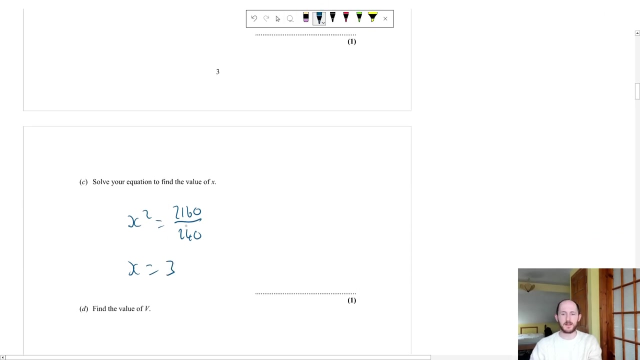 equal to 2160 over 240.. Square root: We're all done So. square root: 2160 over 240.. Three, Look at that Beautiful. And now finding the value of v. Well, v is equal to one over three. 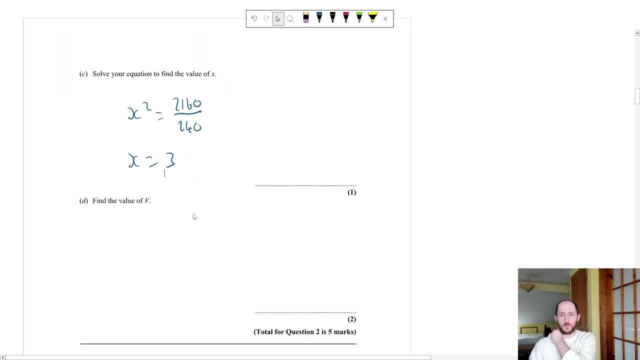 pi r squared h. We know all of the values for everything, so we are all good to go. So one over three pi r squared Well, r was 12x but x is three, So 12 times three, 36 squared. 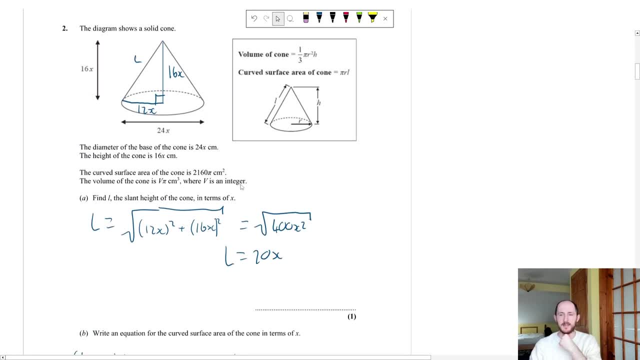 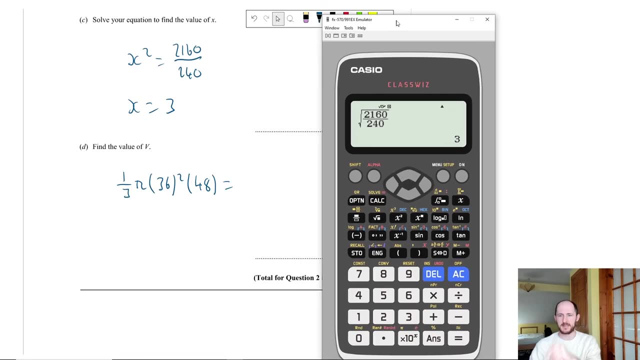 times h, which was 16 times three, So it'd be 48.. It's funny how that last part gives you the most marks, even though it's probably the easiest part, assuming you've got everything else correct, which is obviously a big assumption. 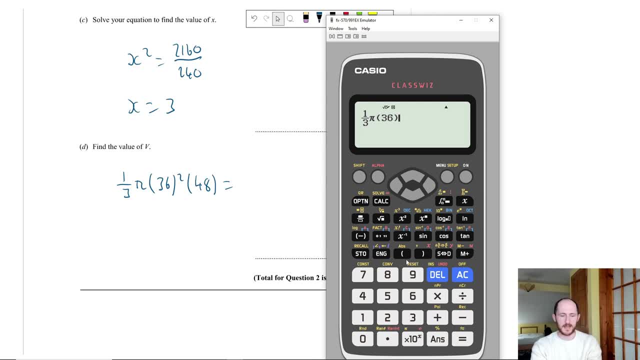 It's not the easiest thing in the world, But again, think about my thought process, how I get to this in general. Damn, that's a big number. All right, It doesn't say to any significant figure, so I'm just going to do it to the nearest whole number: 65144.. 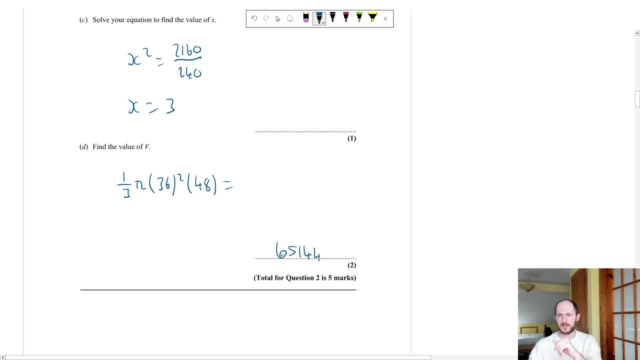 Does it actually say if it's in centimeters or anything? Yep, it's in centimeters. So centimeters cubed. And that's it for question two. Not so bad so far, I think. For question three we have to use. 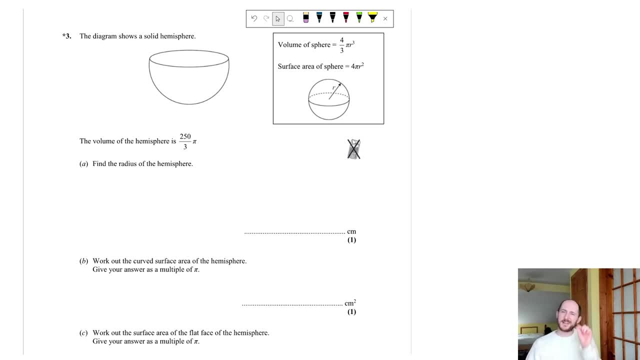 We have to use volume or surface area of a sphere without a calculator, which always makes it a tiny weenie, a little bit trickier. Now the question has been broken up into quite a few different parts in order to help us through it. But again, the thought process. 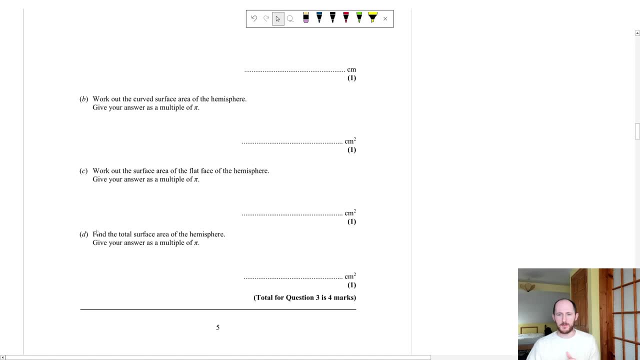 of what counts. which is why I really like these questions, because again, it kind of teaches you. Imagine if you just had to do the last bit: Find the total surface area of the hemisphere. Right, just find the surface area of this. Might be a bit tricky to do. 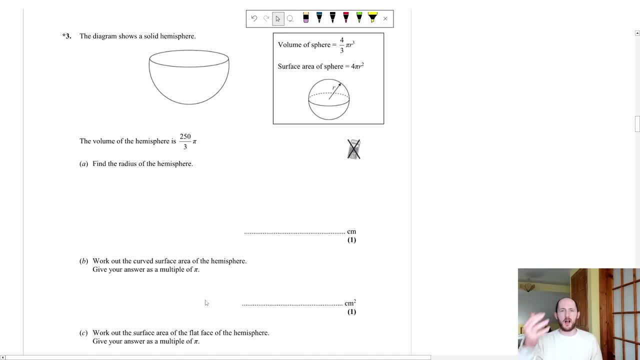 So instead it was broken down into multiple parts to kind of lead you to the answer which will help you develop that grade 9,000.. So that's why this is really good, Even though the individual parts may be easier, the overall. 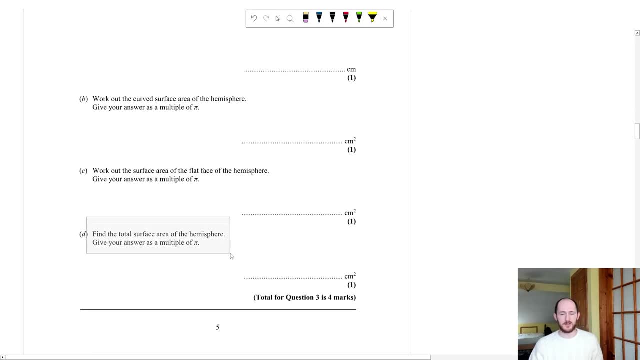 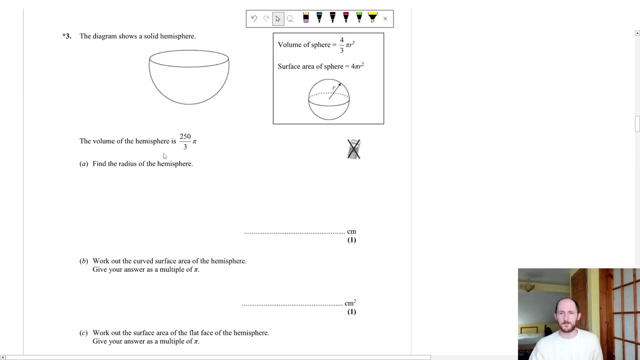 thought process will help, because, if you do get something like this in your exam, you'll know exactly the steps you need to take, because these are the exact steps I would take, which is why I was really excited to show these to you. 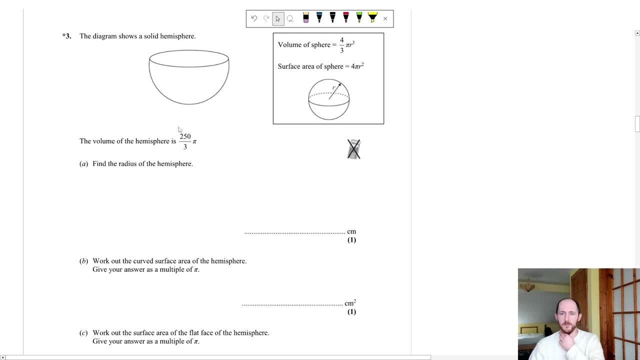 So the diagram shows a solid hemisphere. The volume is this: Find the radius. Well, we don't know right. They've given us the volume and we have the volume equation. However, that's the volume of a sphere. It's not the volume of a sphere, It's the volume of a sphere. 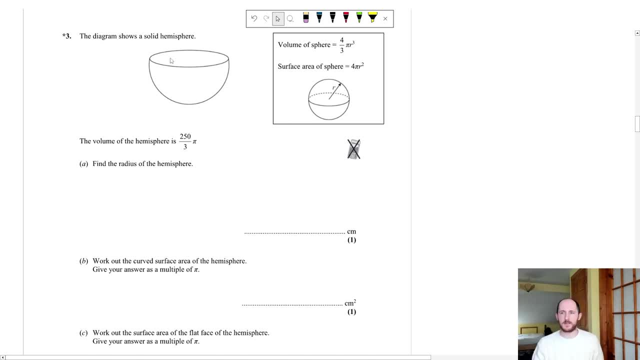 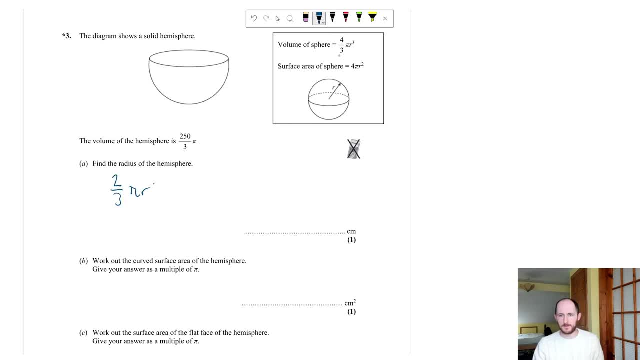 over 3 pi. r cubed equals 250 over 3pi. So I'm gonna show you a few shortcuts. Of course we can cancel out the pi's, but maybe you didn't know that you can cancel out the 3's. 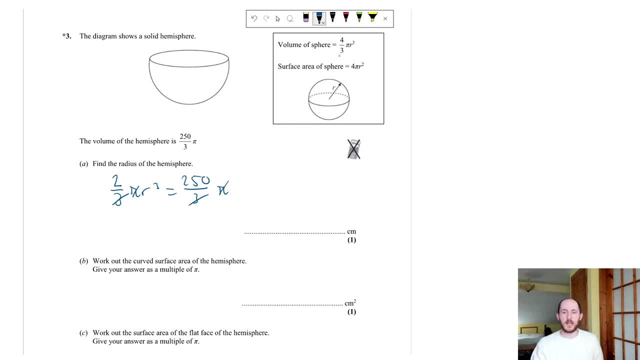 right, Because they're on the same kind of side. They're on opposite sides, but they're on the same. they're both in denominators, on opposite sides, So I can then divide both sides by 2.. So then I get r cubed equals 125, which means r is equal to 5, because you just cube root it. 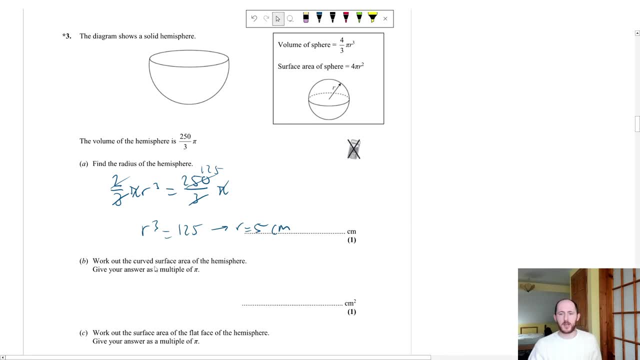 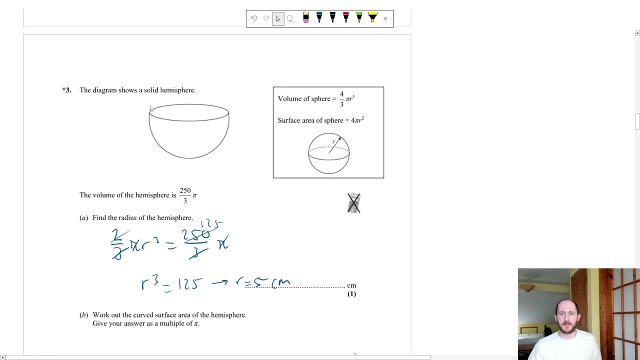 So a few neat little shortcuts there And this is: work out the curved surface area of the hemisphere And this is the really important bit. Whenever I see students answering this: find the total surface area of the hemisphere- they just half this and they say that's their answer. 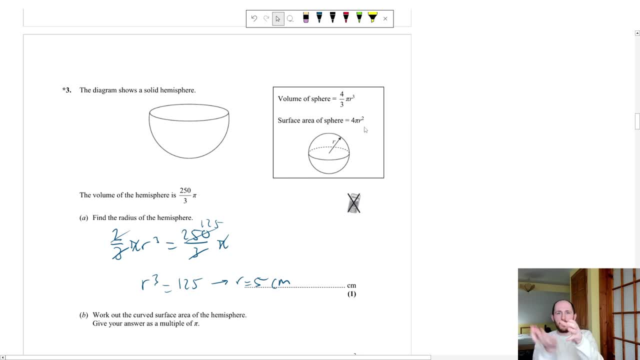 But no, remember, the surface area is the entire area that you can touch. I'm sure the curved bit is going to be half of this. However, you also have the flat bit on top. You would have to add on this pi r squared. 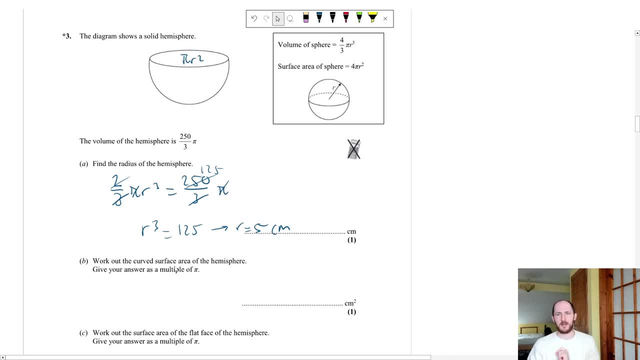 So part B specifies the curved surface area. So now again we're going to half this to make it 2.. So we have 2 pi r squared. So we have 2 pi 5 squared. 5 squared is 25 times 2 is 50.. 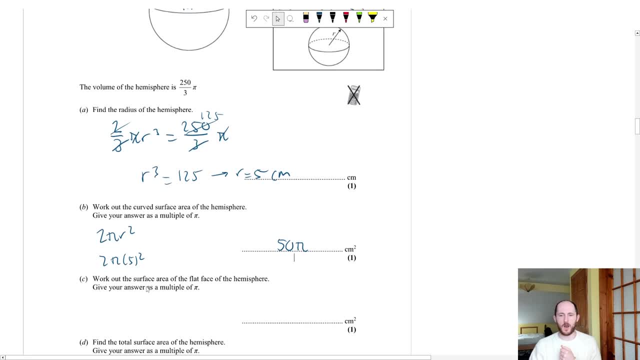 So we just have 50 pi centimeters squared And now it says: work out the surface area of the flat base Again. this is why I really like these questions. They're breaking it down Complicated, hard grade 9 questions into multiple steps which you'll take to do it. 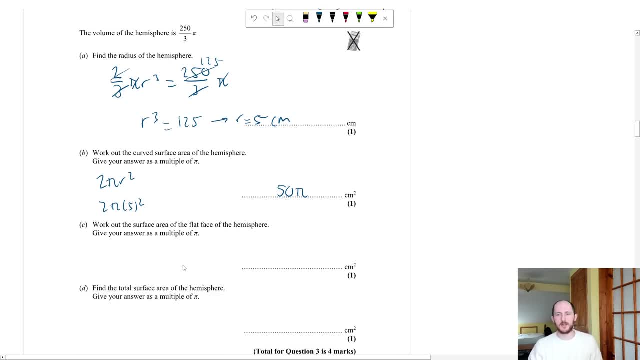 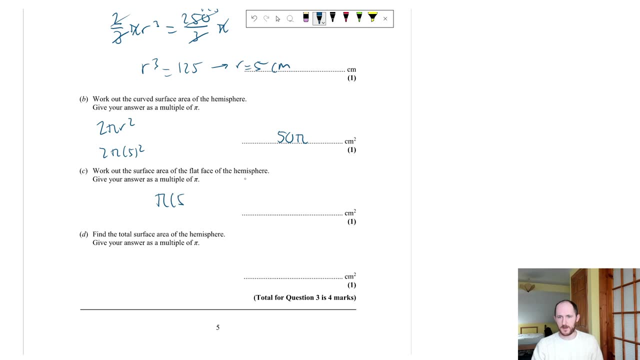 Then you work out the flat face, Then you add it to find the total Beautiful. So again the flat base is just a circle. So pi? r squared, So that's pi times 5 squared, So that's 25 pi. 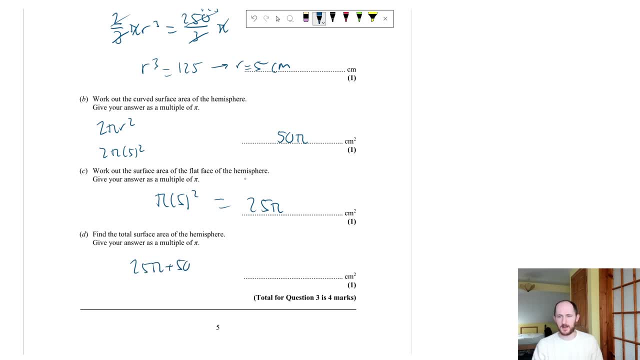 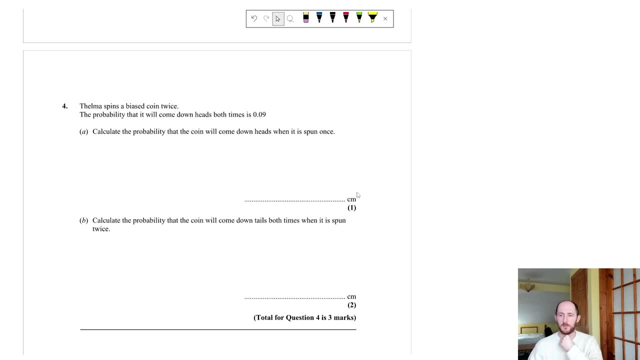 Then the total would just be 25 pi plus 50 pi is 75 pi centimeters squared. Again, what they've done is they've done this. What they've done here is they've split a tricky grade 9 question into two parts. 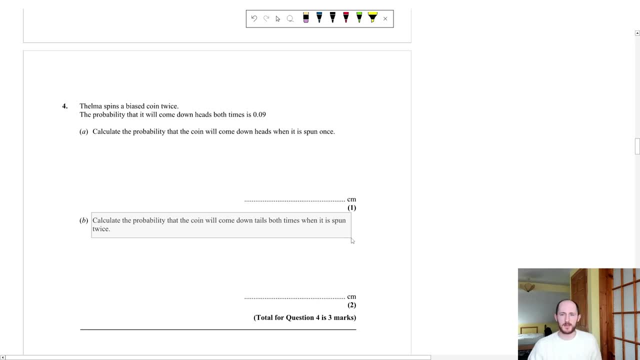 So I've seen very similar questions to this, especially with probability, because it's an interesting way of doing it. So a bias coin is spun twice. The probability it comes down heads both times is 0.09.. Normally the question is: calculate the probability that it comes down tails both times. 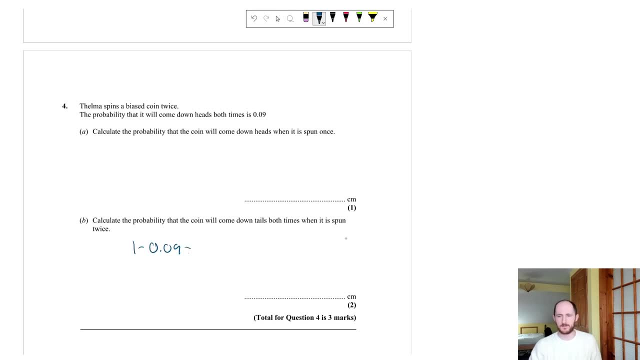 And what I normally see is this: Because if it doesn't come down, you know heads both times- then it must be tails right? Not really, Because it could also have one head and then one tail, Or one tail and then one head. 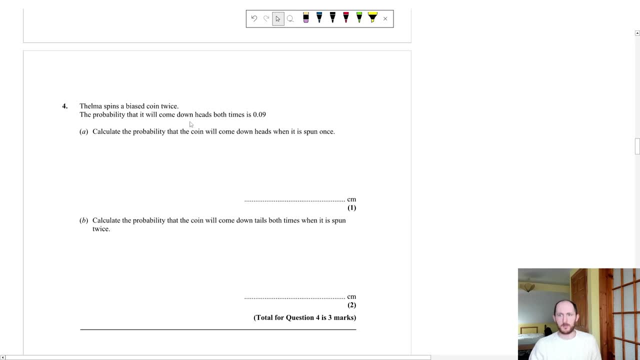 So this is not correct. Instead, what you're supposed to do is know that your probability of heads times the probability of heads should give you 0.09.. So, in other words, the probability of getting heads squared is 0.09.. 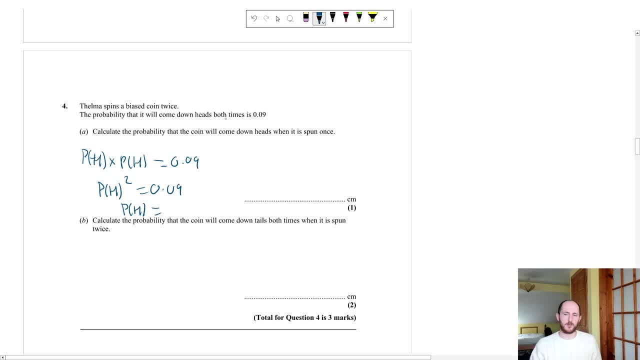 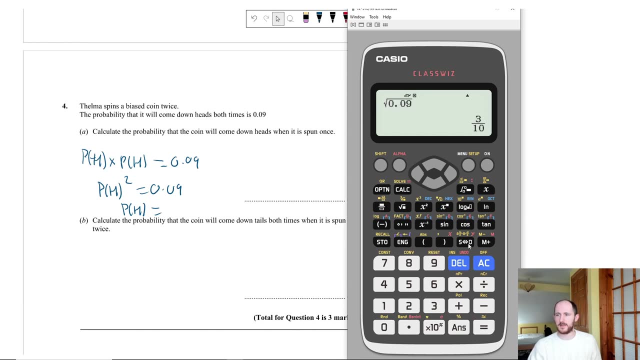 So what's forwarded to getting one head? Well, all you have to do is square root 0.09.. So let's do that Square root. It gives me 0.3.. There you go, Okay. So then, how do you? 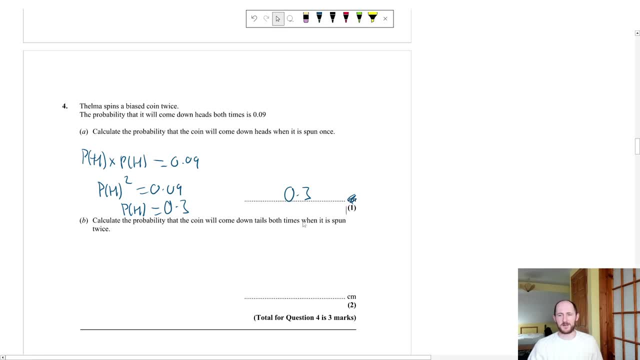 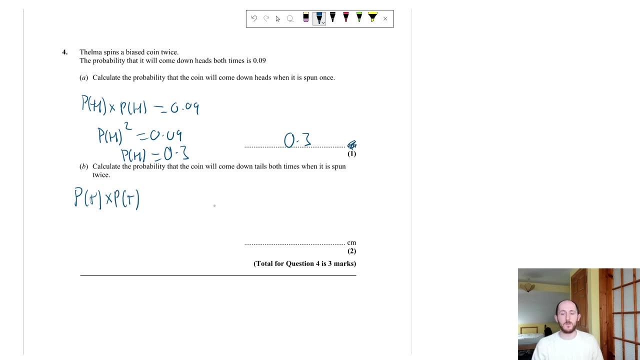 I don't know why the sentiment is there. It doesn't make sense Calculate the probability that the coin will come down tails both times. Well, you'd have to do probability of tails times probability of tails. We don't know that yet. 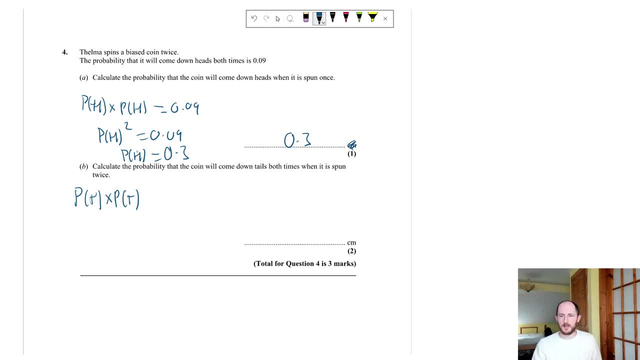 But we know the probability of heads And there are only two options with a coin. So the probability of getting tails once is just 1 minus 0.3.. Because it's the only other option, The 0.7.. So the probability of tails times the probability of tails would be 0.7 times 0.7, which is 0.49.. 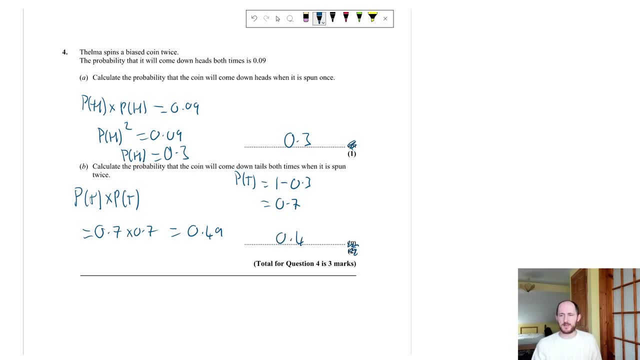 So again, I don't know why I crossed out the wrong thing there. It would be 0.49 instead of the kind of normal typical mistake that I see. So again, that's why I love the fact that they broke down these questions so nicely. 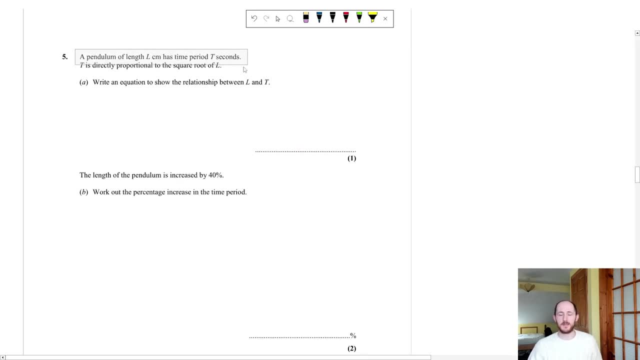 Potentially a question you've seen before. So the pendulum length L, has time period T. T is directly proportional to the square root of L, And then it would say: you know, it's increased by 40% Work. We've got the percentage increase in the time period itself. 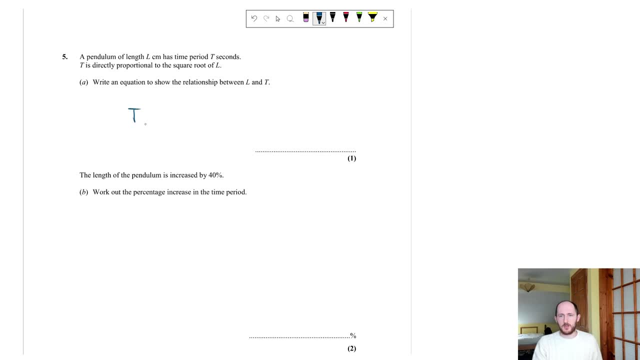 So here's what you do For the equation: you would just write, And that's it. You do not need the K root L. technically You can leave it like this: The length of the pendulum is increased by 40%. Well, that means of 1.4 L, right. 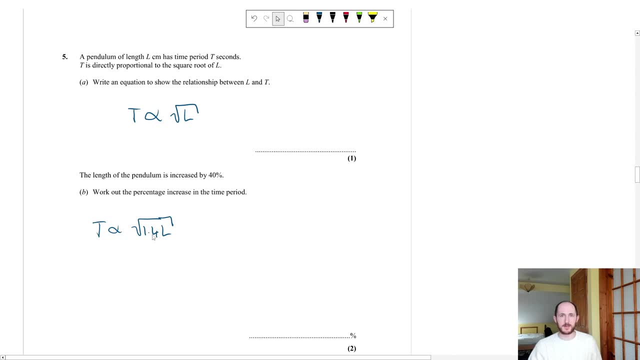 So if we increase L by 40%, that means this value Is going up by 40%. a 40% increase is the same as 140%, which is the same as 1.4.. So all we're doing is work out how many times bigger T will be. 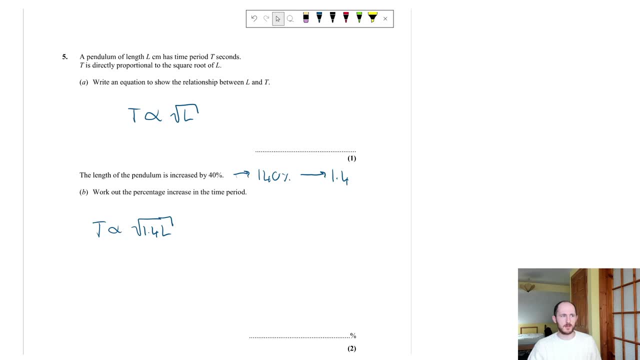 So T is proportional to one with the square root of 1.4.. So all I do is I take the square root of 1.4 and I get 1.183. blah, blah blah. So that means T is going to be 1.183 times bigger. 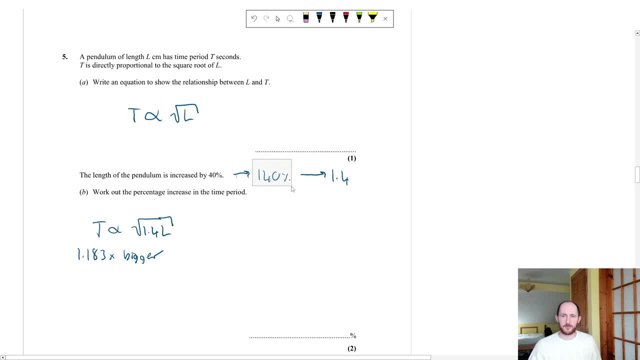 So what's the percentage increase? Well, from here I went from the percentage to the decimal, So now I'm going from the decimal to the percentage. So that is 118.3%, which means it's an 18.3% increase. 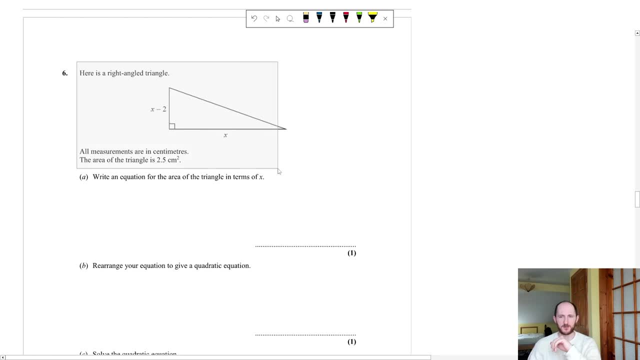 That's all. This is actually quite a long question. So it's right angle triangle and they give us the area And, if you notice, this would normally be the actual question. Maybe a six marker find the perimeter based on this. So again, the way it's broken down is really really nice. 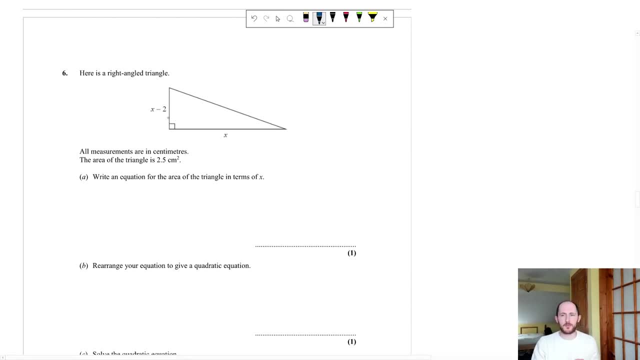 If I wanted to find the perimeter of this triangle, what do I need? Well, I need all three sides, so I need to work out this side here, And I know you do that with Pythagoras, But the thing is, I still don't know what X is. 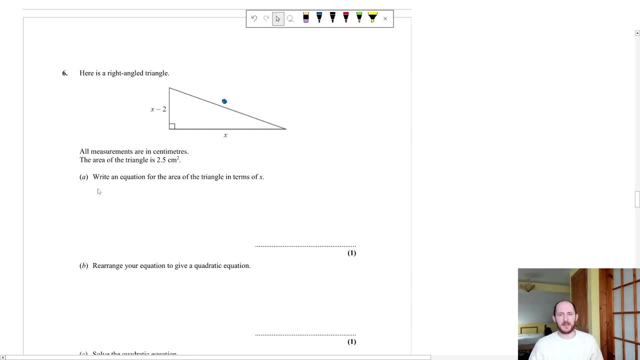 So then I'd have to use this area of a triangle thing here And again this: these questions really take you through nice and neatly, Exactly how you would answer a question like this. So you first find an equation. So half base times height. 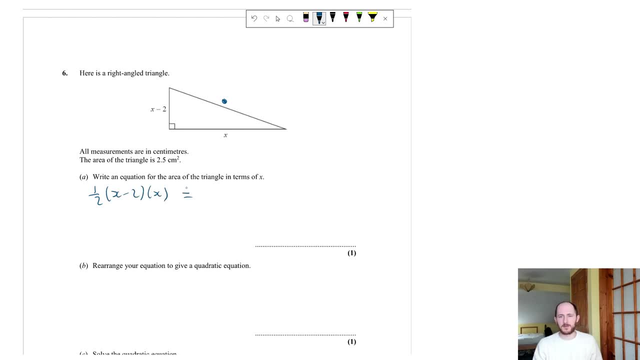 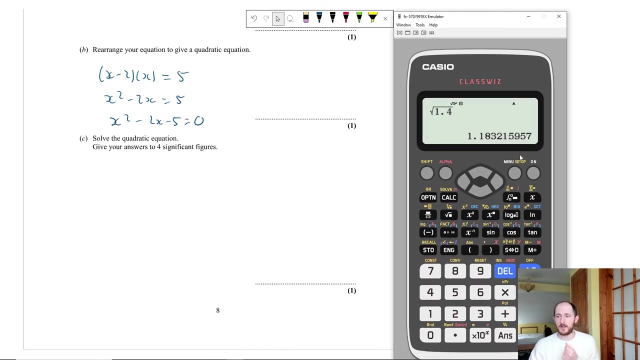 Not too bad so far. And then it says: solve it. giving us to four significant figures, which means they're probably- I would be tricky, I would use quadratic formula or, if you have this calculator. 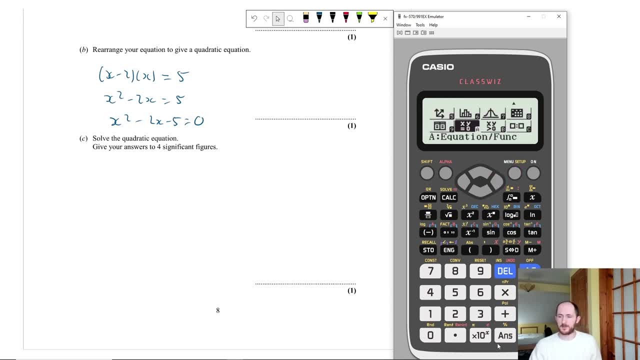 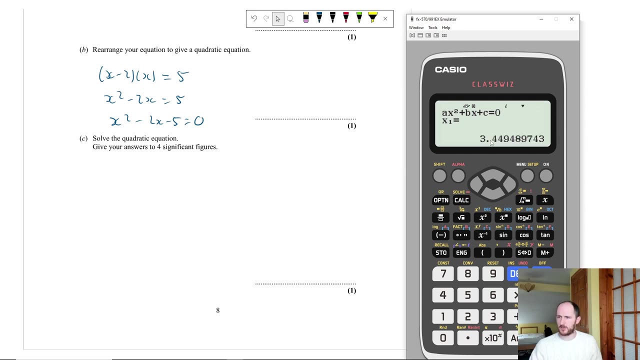 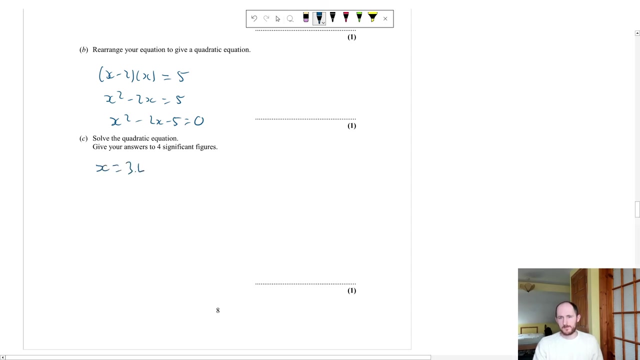 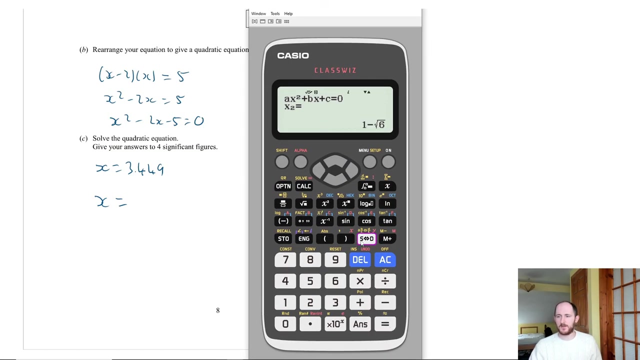 go to menu, go down twice. equations slash, func, polynomial, polynomial, degrees 2, and you're just subbing the value, So 1 minus 2 minus 5.. And we get 1 plus root x. this is to 4SF, sorry, So 3.449.. And then of course we have the other solution, minus 1.449.. 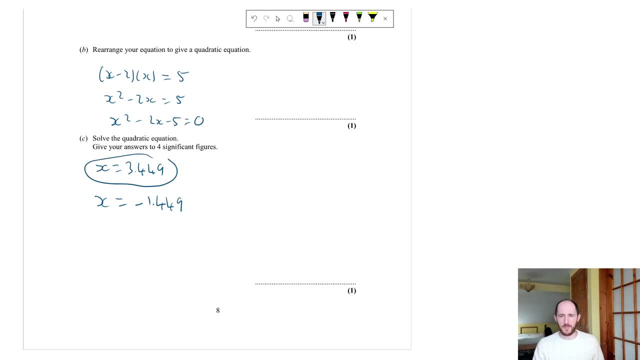 So of course the answer here is going to be the top one, because these are sides. So of course we can't- We can't have a negative length, right? If I asked you to measure something that's negative 5 centimeters, you'd look at me like I'm weird. So now we find the length of all the three sides. 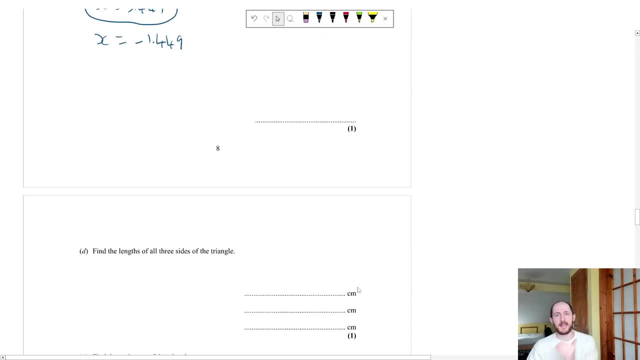 then we find the perimeter Really nice way of laying this out. In fact, I would go so far as to say that if I were answering just part E straight away, I would lay out my work exactly like this in order to get the six marks. There's no coincidence that the number of parts is almost. 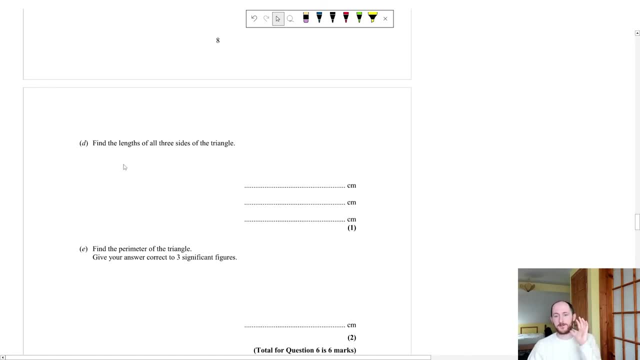 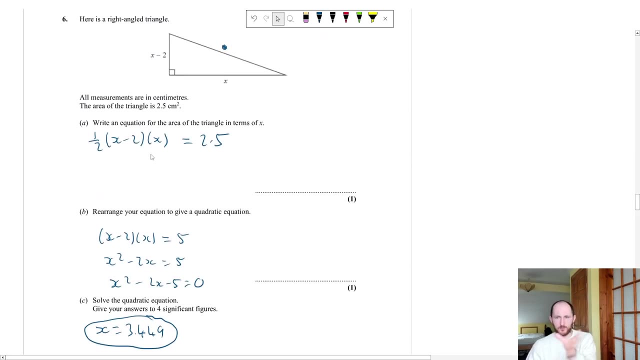 equal to the number of actual marks you get. in the question It's five parts and we get six marks And if you notice, the last part is worth two marks anyway. So again, you would write an equation, solve it, do it? So I know this may seem really basic to you. 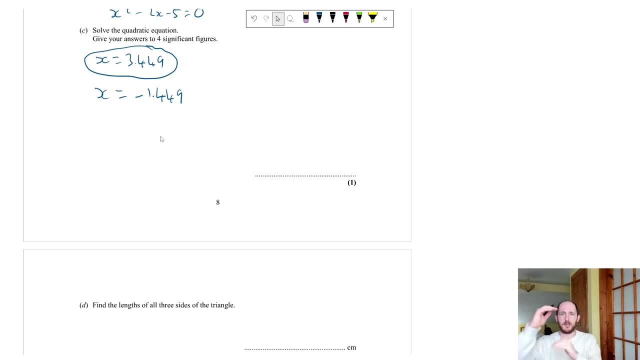 but that's kind of the point. If you make a really complicated question and you break it down and break it down, and break it down into one-mark questions, you can really see how easy questions like this are. And that's what I find really valuable about these papers. I will put the rest. 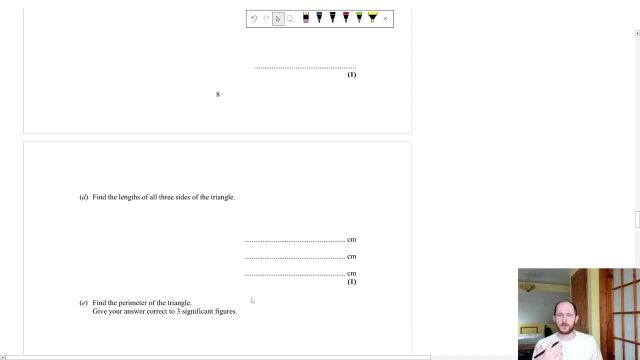 of them in the description for you to go through, because they help you answer those grade 9 questions. It's really, really useful. So the length of all three sides, so 3.449 minus 2 would be 1.449.. The side down here is just x, so that's 3.449.. And then the third side is Pythagoras. 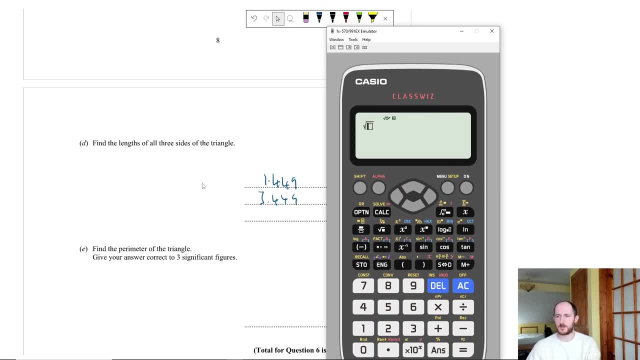 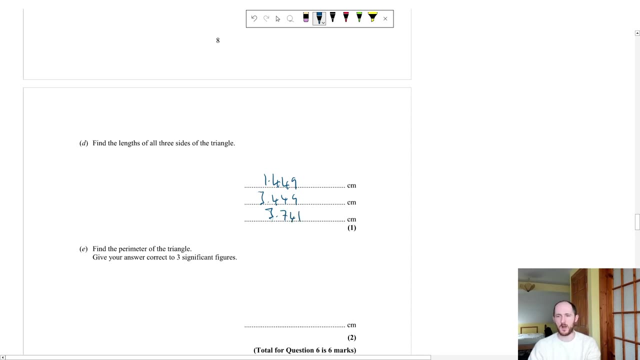 so we're going to go menu number 1.. So it would be: square root, 1.449 squared plus 3.449 squared. All square rooted gives me 3.74.. Subtitles by the Amaraorg community: Actually, we should probably give it to 4SF, so 3.741.. Then all you do is add them all up. 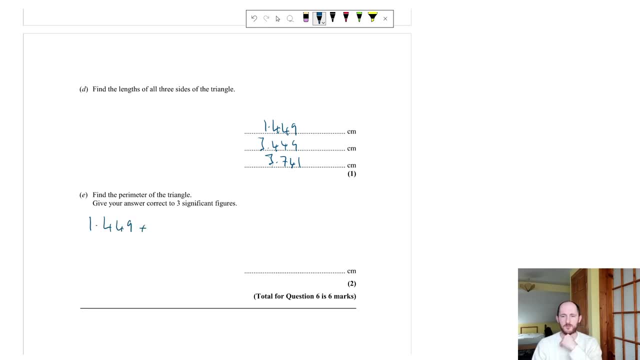 And if you look how simple that is And you know what else I really like about this question as well is sometimes I see that students make rounding errors, but they're not the rounding errors that you think. It's not that they round incorrectly, It's that when they find the lengths 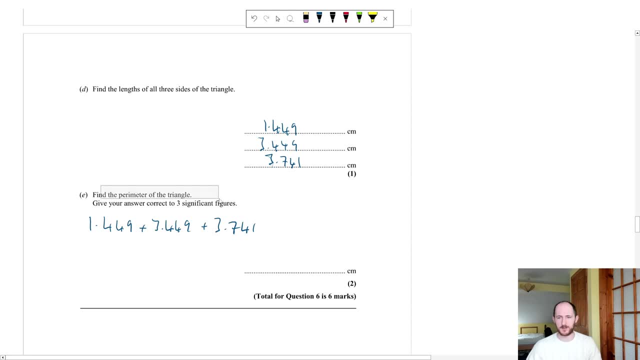 they might round to just one decimal place, which means their answer is actually wrong, or they round to two decimal places or whatever. But if you look at the question it will say round to 3SF. That doesn't mean that you're. 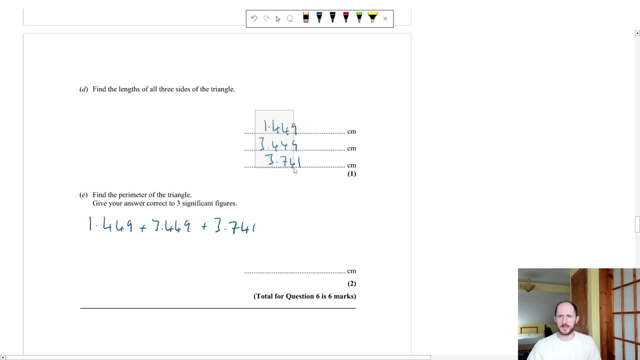 working out it should be to 3SF, Because, if you notice, if I round this to 3SF and then I don't round to 3SF, I'm actually going to get slightly different answers. So the other thing I really like about this is that they tell us 4SF in the question when they broke. 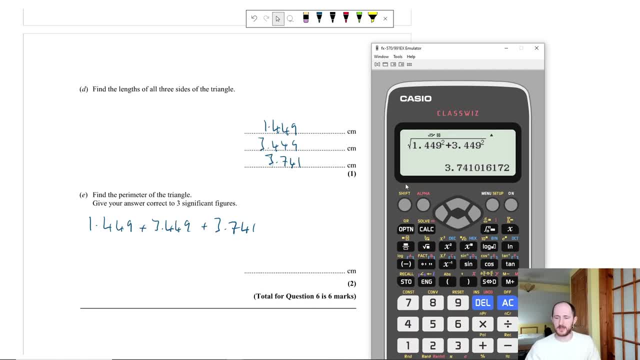 it down, which is very, very useful, Because, again, I do notice rounding errors with some people. Generally, and here's how I do it is: if the answer is to 3SF, I will give my working out to 4SF, And then I'll round to 3SF, And then I'll round to 3SF And then 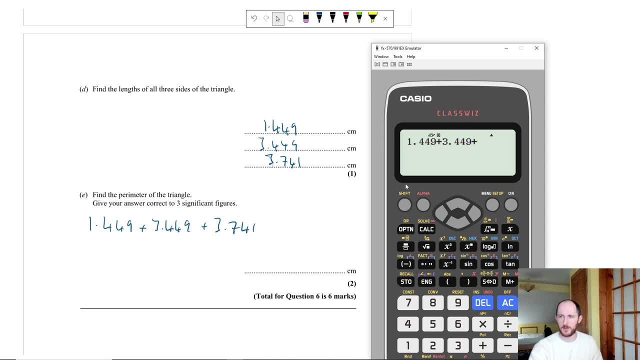 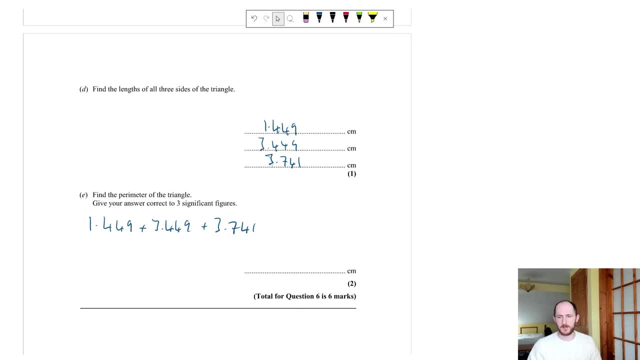 if it's to two decimal places, I'll do my working out to three decimal places. That way I can be sure that when I round it won't make a difference But 8.64.. If you round them before, you might find that you actually get a different answer, which would be kind. 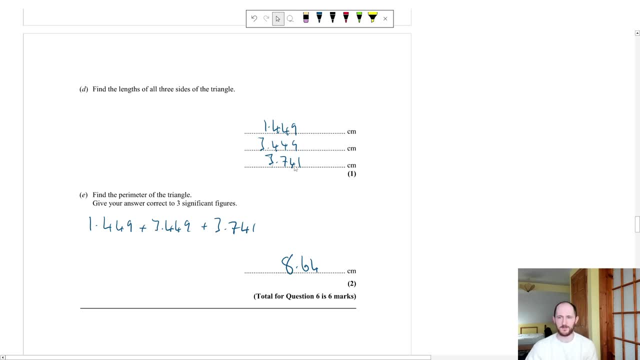 of annoying. In fact, if you notice, it'd be 5,, 5, and 4, which would actually give you 8.6.. Actually, it might be okay for this question, But again, in some questions it. 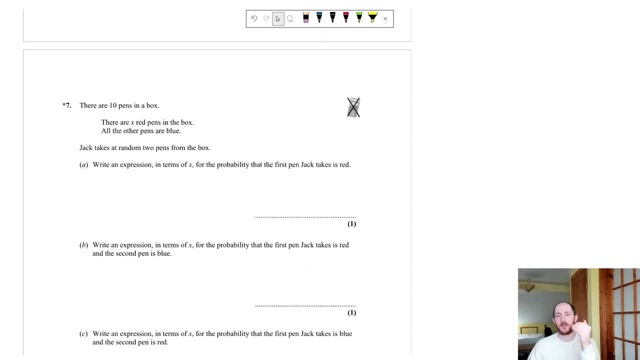 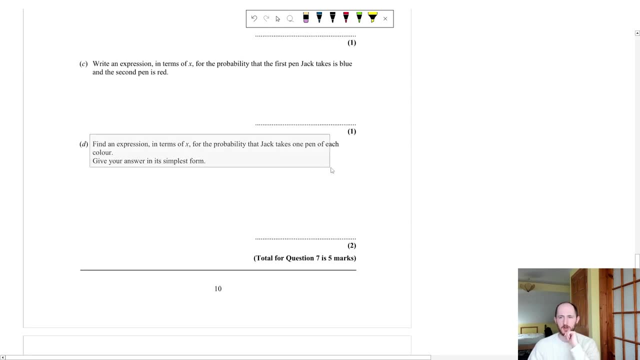 will actually give a slightly different answer. Another grade nine question: 10 pens in a box. There are X, red pens, other pens are blue. Jack takes two random pens. Find an expression for the probability he takes one of each colour. Such a common question. Probability will come up in your exam And there is such. 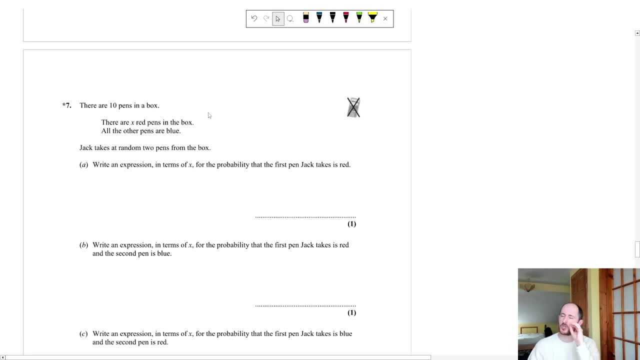 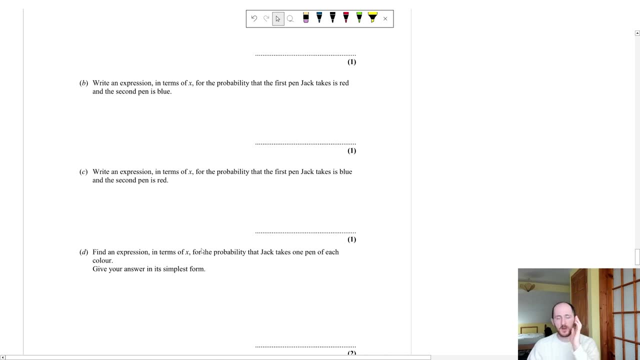 a high chance that it would be something like this where there's algebra involved. Such an unbelievably high chance- I would say it's somewhere in the region of 80%- that something like this will come up. It's really common. So I'm really working this down again. I know I'm really harping on about this, but 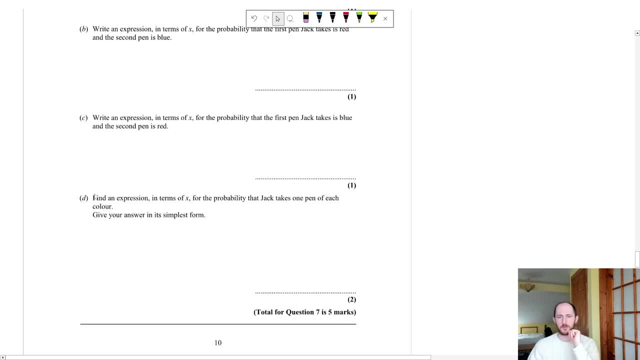 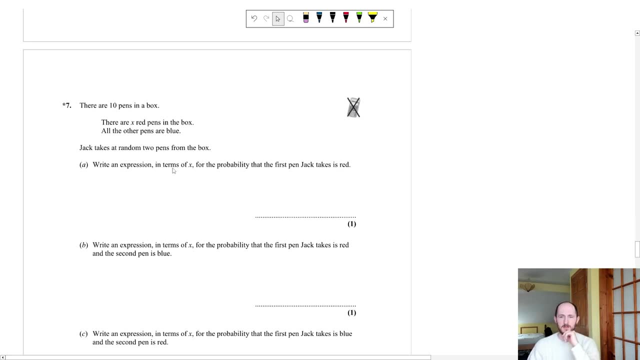 these questions really really break it down so good, Because just doing this would be very tricky for some students. So what are they doing here? Well, write an expression for the prob- in terms of X. the probability of the first pen Jack takes is red. Well, 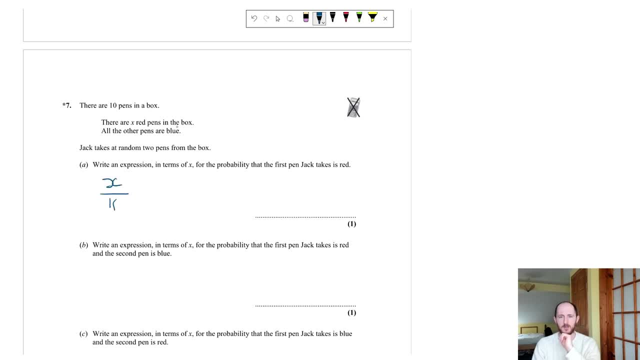 there are X red pens and there are 10 pens in total, So X out of 10.. That would be my first step. two, Then, the probability that the first pen Jack takes is red and the second pen Jack takes is blue. Well, it'd be X over 10.. And then, because we've got two steps, 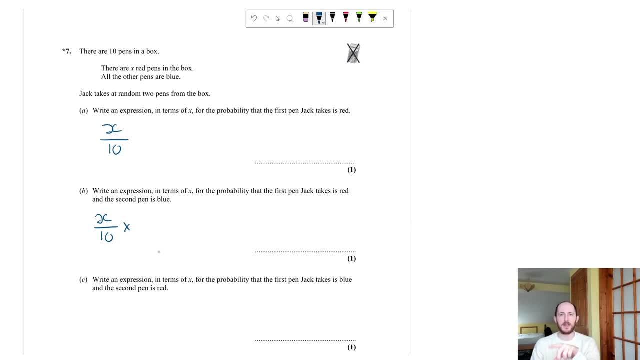 now it's, AND we do times. the second pen is blue. Now, if there are X red pens, how many blue pens are there? Well, it says the rest are blue. So that means there are 10 minus X blue pens. So it'd be 10 minus X, because we haven't taken out any blue pens. 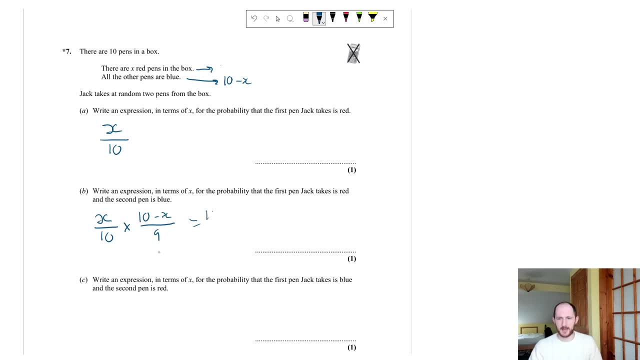 over 9.. And you could simplify this to make it 10X minus X squared over 90.. Just so you know, my method for this question is, of course, X minus X squared over 90.. So I'm just going. to write this down. So I'm going to write this down, So I'm going to write this down, So all right, So I'm going to do that, And then I'm going to write this down. So. 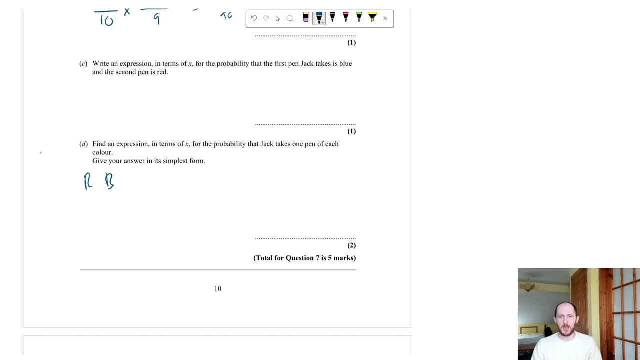 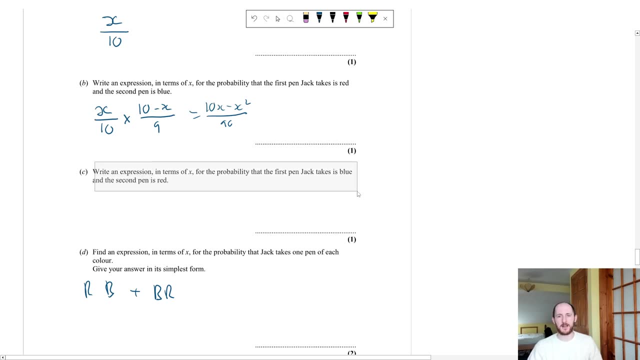 if I write the probability of that, we take one of each colour. You're going to do the probability of red and then blue, plus the probability of blue and then red. So if you notice, we've already done the red and then blue, And now look, It's blue and then red. 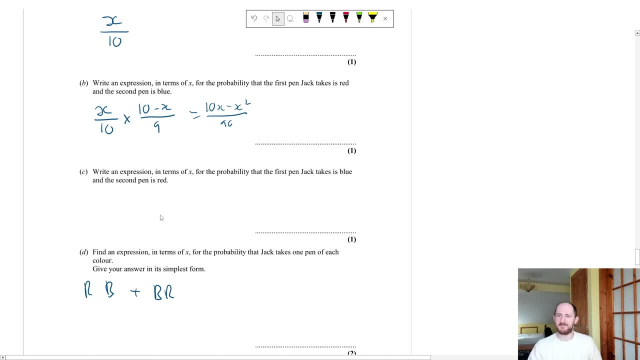 But how easy are these individual parts? I know I keep saying it, but it's a really really good way of breaking it down And I actually have a video coming up soon about how to actually revise different subjects And I would say this is an exceptionally good 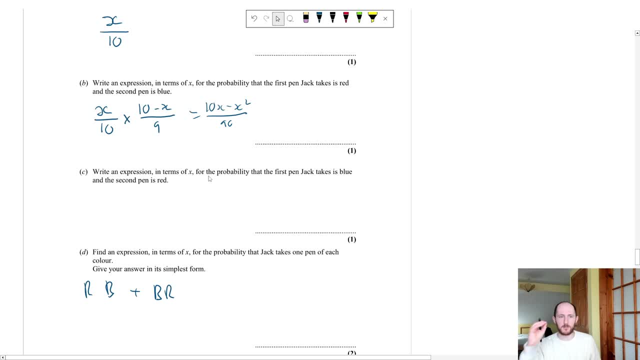 way Where what you do is you take big question, starting with the number, and then you divide it by the number of the questions. So I'm going to write this down. So what happens? questions and you break it down simpler and simpler and simpler, until you have someone. that's. 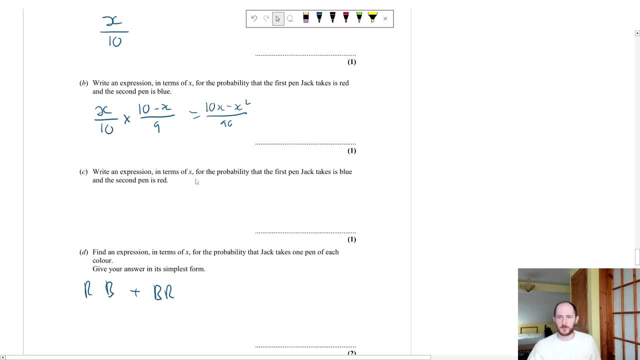 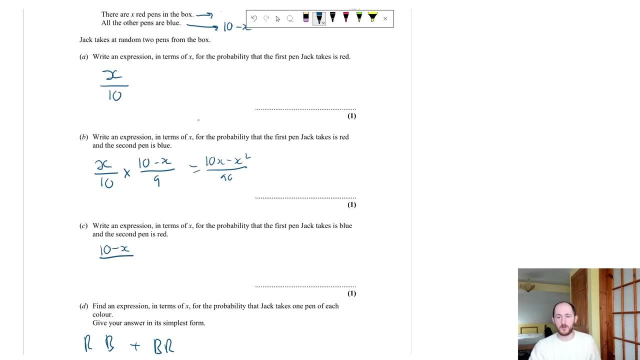 far less experienced being able to do it for you as well. so expression for blue and then red. well, blue again is 10 minus x over the total, which is 10 times then red. well, there's gonna be x red pen still left over 9. expand this, you get 10x minus x squared over 90. find one of each color. well, 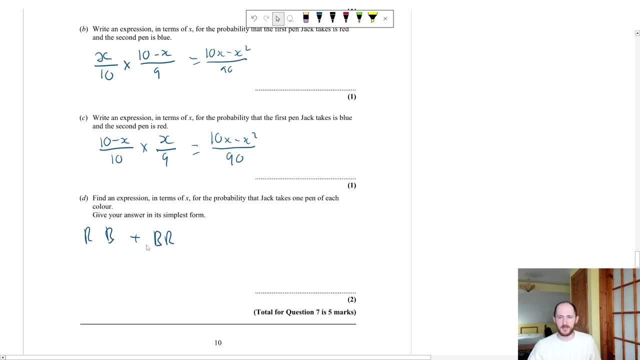 now all we need to do is add those two together, because we've worked out the individual parts. so again, it's the same methods i teach. it's just broken down into different questions, which is amazing. i love it. so we have 10x minus x squared over 90. add 10x minus x squared over 90, so the 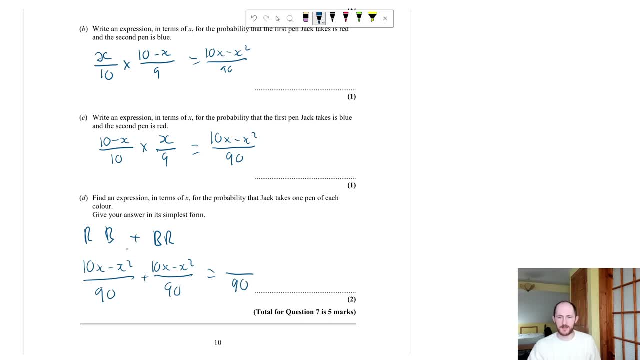 denominators stay the same. when you're adding fractions, you seem to make sure the numerators are the same. sorry that you need to make sure the denominators are the same and then they stay the same, but the numerators you add so be 20x minus 2x. 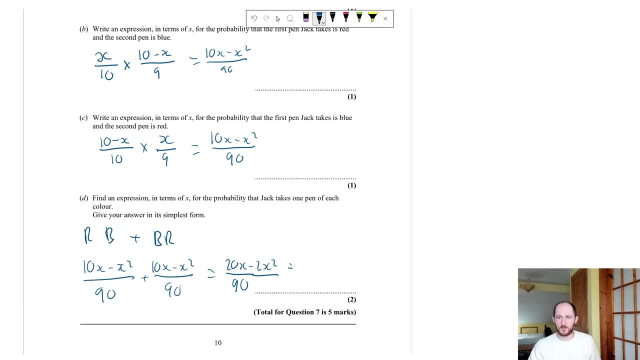 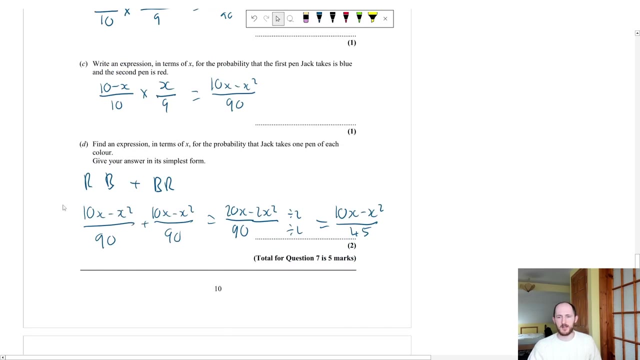 squared. now. simplest form: i can actually divide the top and bottom both by two. so that would be our simplest form would be 10x minus x squared over 45. that would be your simplest form. so they really made that five marker a really tricky five marker quite simple. i've actually done a question. 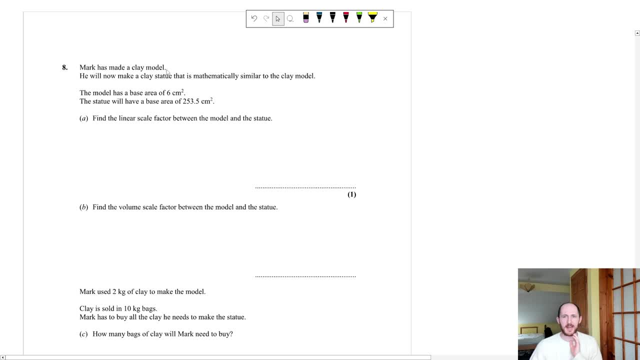 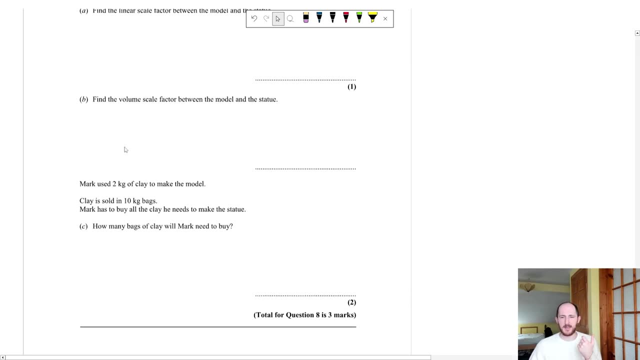 very similar to this in one of the last um grade nine questions. so the clay model and he's making a mathematically similar uh statue to the clay model and he gives you the base area and basically they say: mark used two kilograms of clay to make the model. it's sold in 10 kg bags. 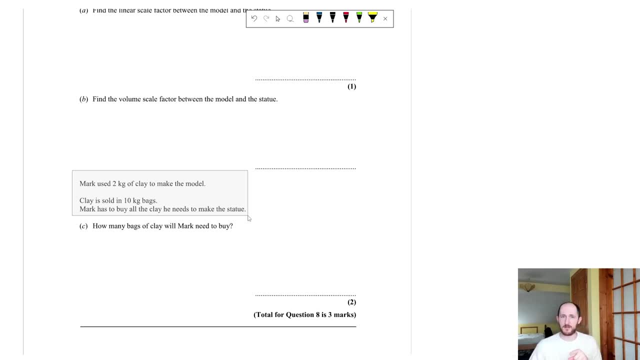 how many do you need to make the statue? the idea is you need the volume scale factor, because volume would change. what the actual mass you need is because, again, uh, density is mass over volume. so in this case, uh, sorry, if you want the mass, it's density times volume, because the density is the 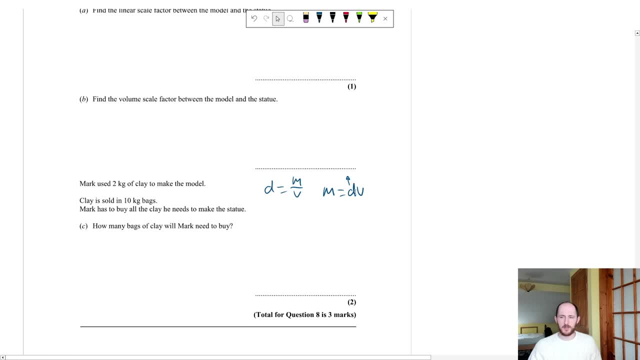 same because it's they're both the same material. it's the volume that is going to change the mass and, yeah, you jump straight into it in order to do the full thing. i actually think this would be a four mark question, not three. i think they missed out putting a one mark here, but whatever, um, and. 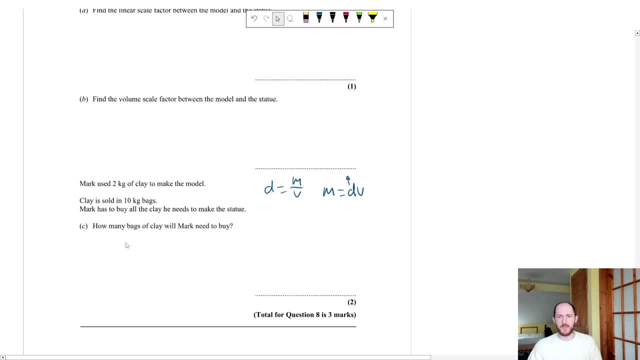 this is exactly what i do, so find the linear scale factor, find the volume and then do it. so it's again broken down nicely. so if i were answering this question, first thing i would do is find the linear scale factor. so we have the the area scale factor, which would be: 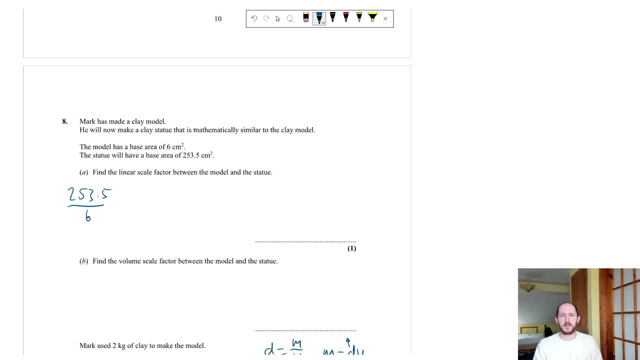 two, five, three point five over six. now the link between length to area is: you're going to square the length scale factor and to get to volume- i don't know why i didn't put that there- you would cube the scale factor. so in order to go from area back to length, we are going to square root the scale factor. that will give us. 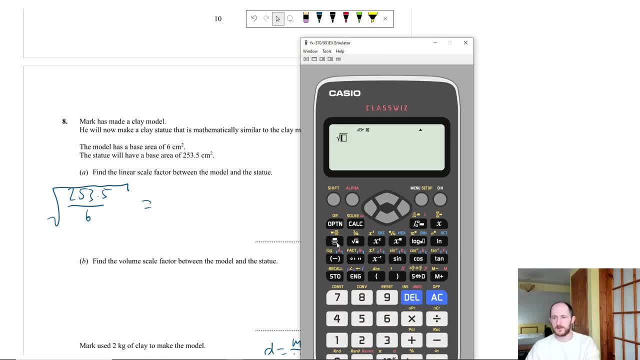 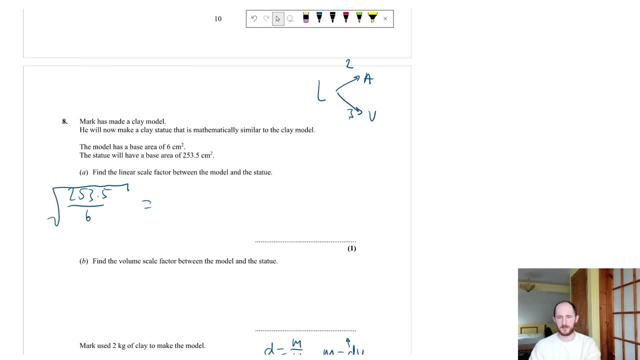 called the linear scale factor or the length scale factor. two, five, three point five over six, 13 over two, that's a nicer value than i thought it would be. then we need to go up to the volume scale factor because, as i mentioned, with mass, it's the volume that impacts the mass, not the area or the length. 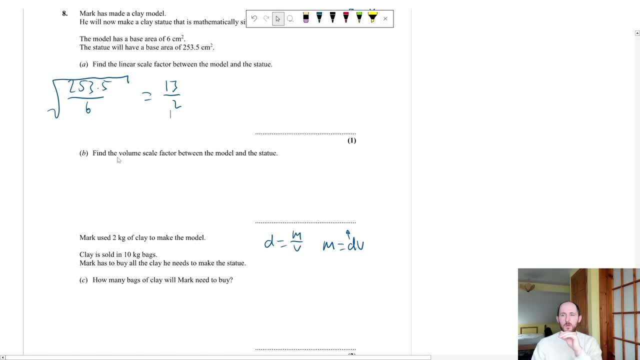 although area and length are linked to volume. so well, again, to go from length to volume, you'd cube it. so you do 13 over 2 cubed. so i might just do answer about three and these are literally the steps i would take: two, one, nine, seven over eight. 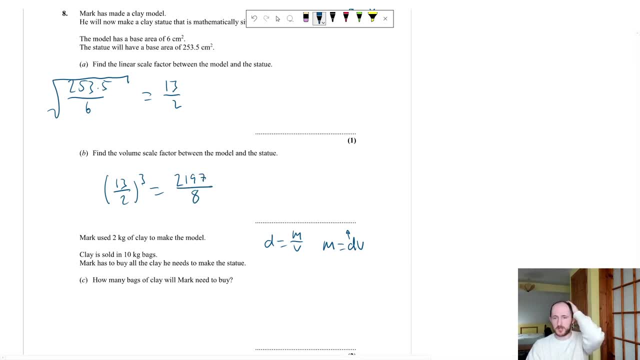 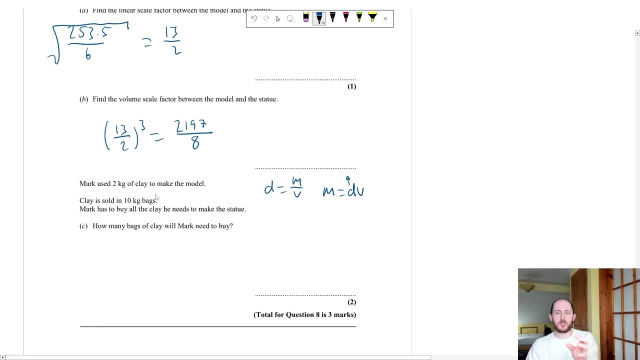 over nine times the ratio of two, two, two times mana, with your left hand to your right hand to do Зап. this is the requirements why this entry is not suitable for possibly both exercises. then it says: mark used two kilograms of clay to make the model. clare sold in 10 kg bags. he needs 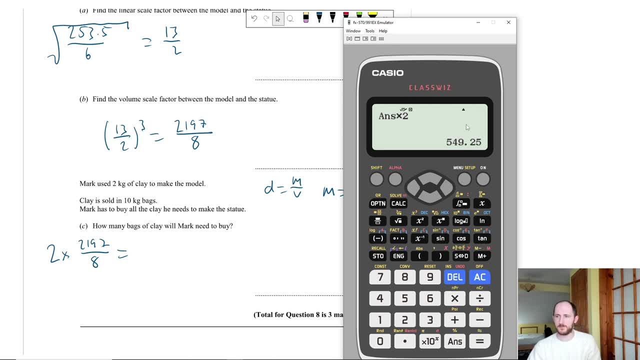 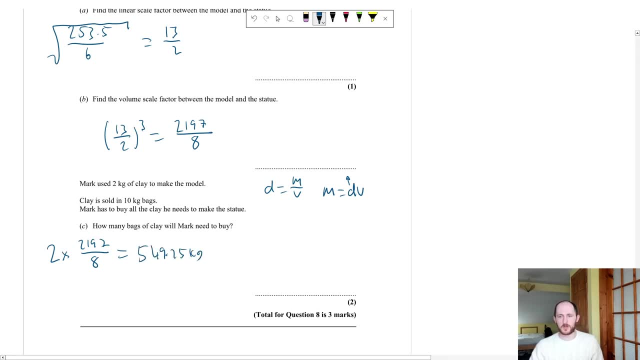 to buy all of it. so if you use 2 kg for the model, 549.25 kilos of clay, and of course all we need to do is divide that by 10 to get the number of bags he needs, which is 54.925.. 54 bags won't be enough, so he must have 55 bags and obviously this: 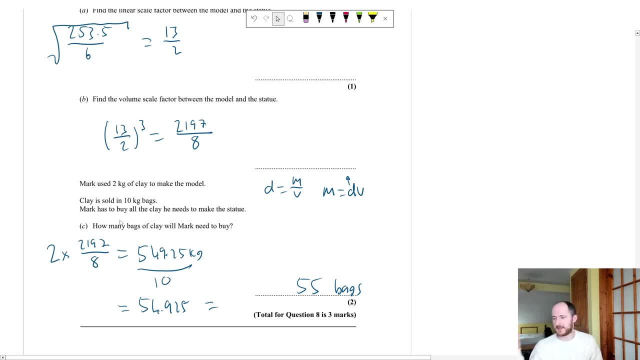 the extra mark they could give you there is, you know, bags cost £5.99. how much does he spend? but again, we're doing his times in that. What I find is one of the biggest issues with these students that are really good mathematically: they know all the processes, they know how to time. 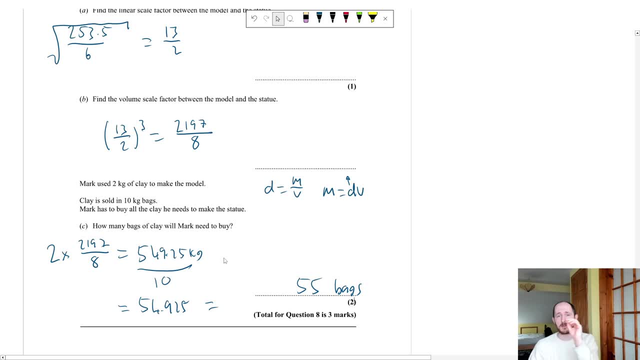 stuff, divide stuff. they know algebra, they're good, but the problem when they come to the exam is the question's like a paragraph long and they don't know the steps. so imagine if I said, for example: I added on to this and I said: how much money would Mark have to spend to buy all 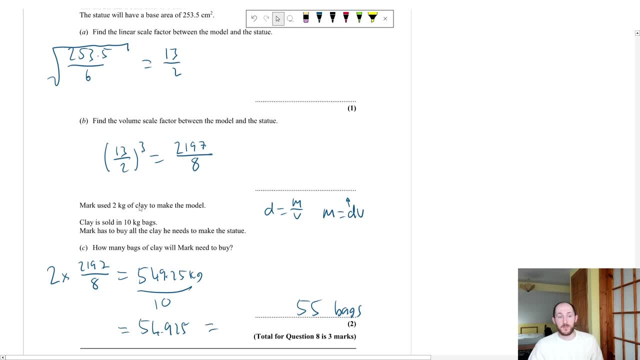 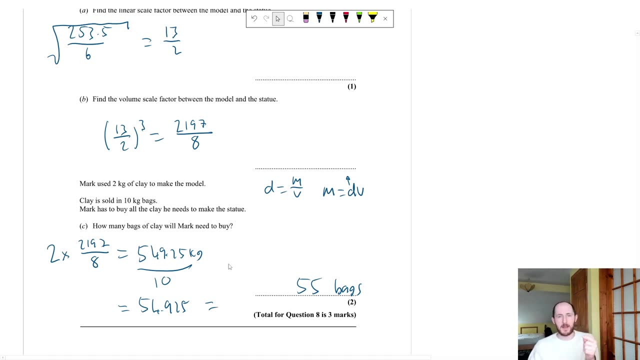 the clay he needs, and I didn't give you these other parts. that's difficult, right? because it's like okay money. well, I need to know the number of bags, then I need to know how much mass, then I need to know- and you have to work backwards- The reason why I like these questions, especially when you're 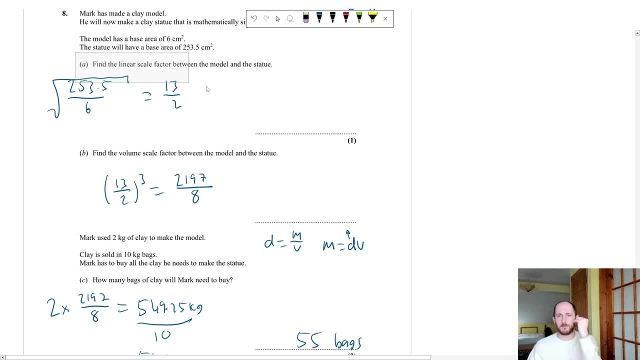 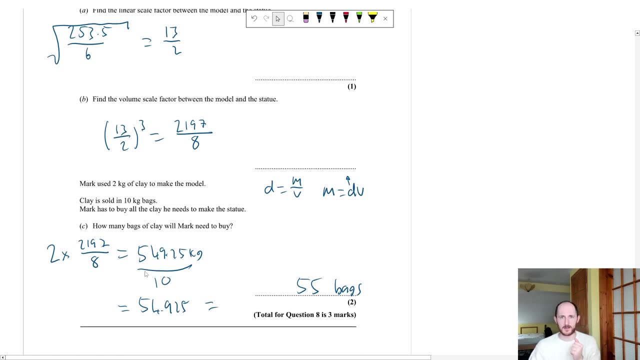 training, which is what you're doing right now. you're training is. it builds the thought process for you and hopefully you can see the link now between going from here all the way to the answer and that's the really valuable skill. so most students when I say to them: okay, what do we need? 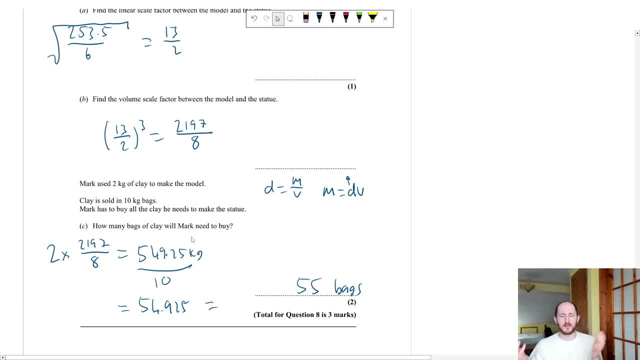 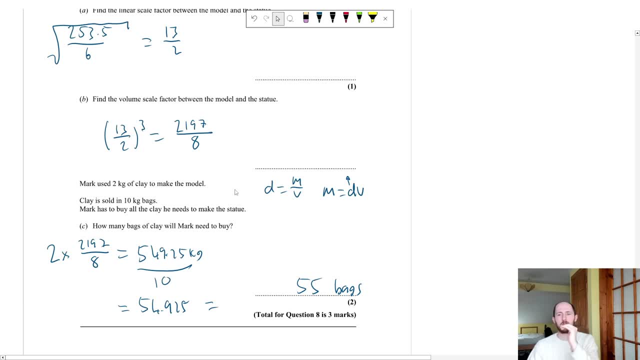 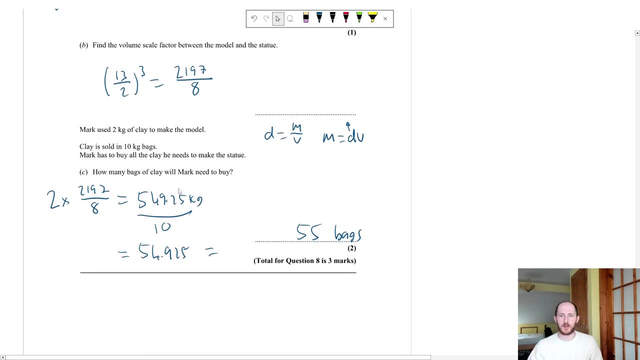 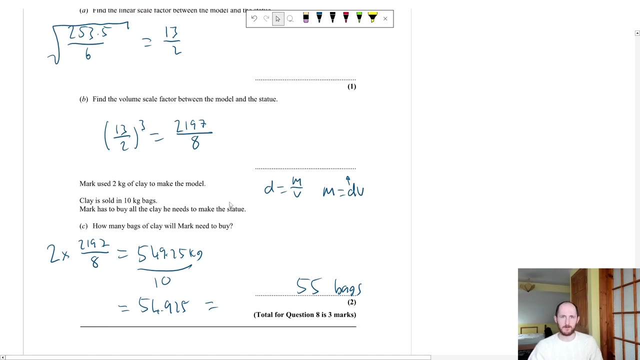 8 and 9s. I'd say you need to be able to break down big questions into small questions like this. it is the most valuable skill you'll have. so it's like: okay, what, what's the end goal and how do I work backwards from there? working backwards generally is much harder than working forwards. 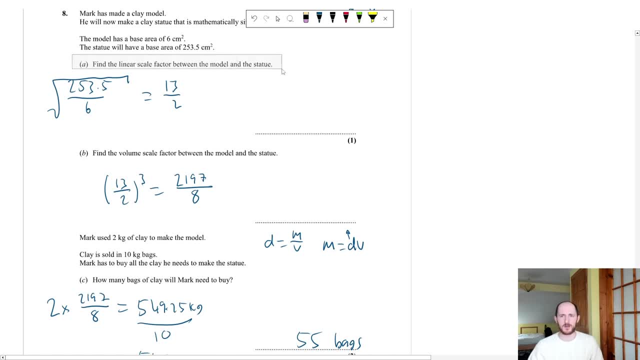 if I- and again I'm willing to bet you guys sitting there probably saying these questions are easy, how are they grade 9? they are grade 9 questions broken up into multiple parts, which simplify it, and that's the main thing that stops you from getting a grade 8 or 9 is your thought process, not the maths. if you, 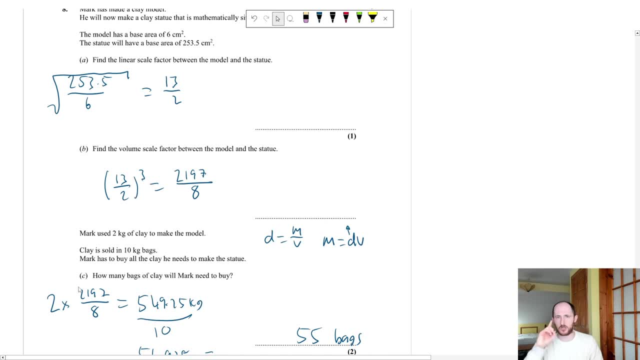 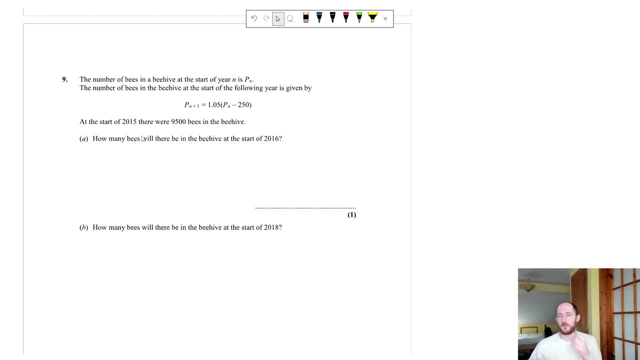 find these questions individually easy, then it's just your thought process you need to go through, which is why I've done these grade 9 videos- this is good, old-fashioned iteration, repeated percentage change, whatever you want to call it- and and which is why they haven't managed to simplify the 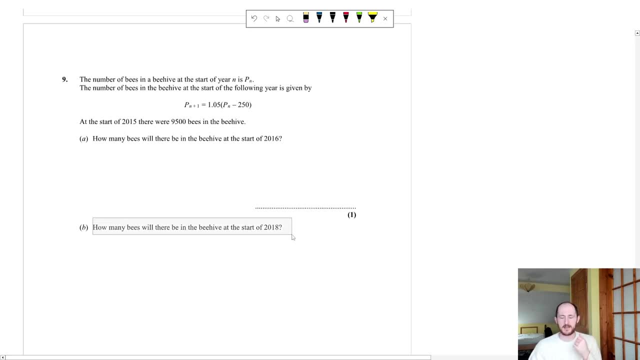 question that much. this is really common. how many bees to be in 2018? I'm going to show you my method. okay, the reason why it's repeated is because it's a good, old-fashioned method. it's a good, old-fashioned method. it's because this equation is going to repeatedly keep subbing in new values. so here's. 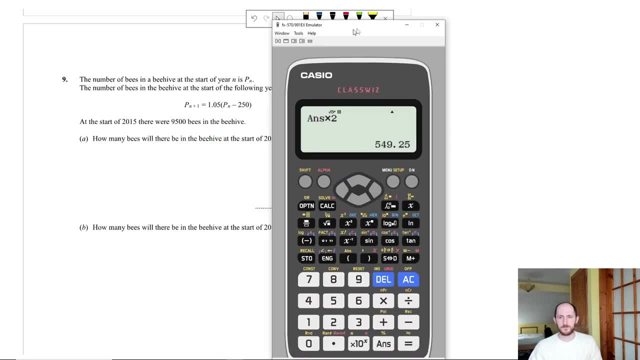 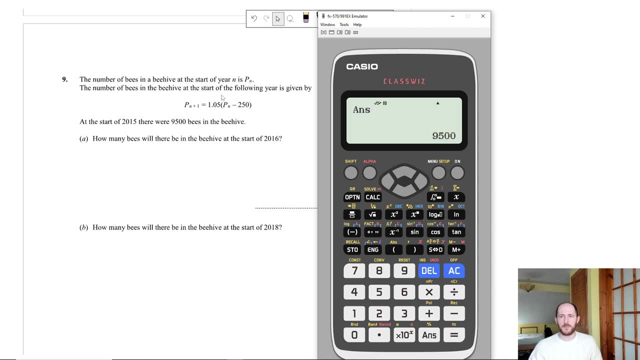 what we do. you take your initial value, 9500, and hit the equals button. that is now your answer button. then you rewrite this exact equation, but instead of pn you're going to put the answer button. this is how many bees there are in 2016, 2017, 2018. that's your answer. 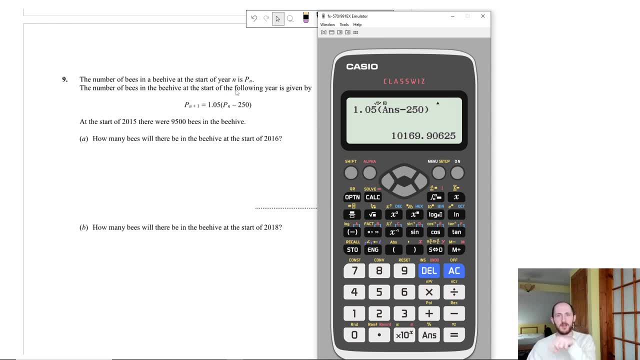 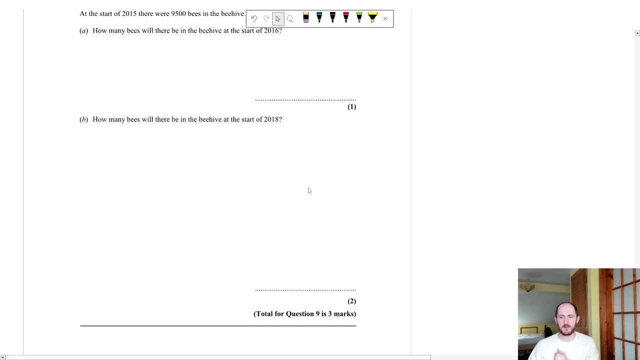 because what it's doing for me is resubbing in the value automatically. really clever, and obviously you'd round up so 10,170. that's it for three marks. absolutely insane. the only thing I would say is: do not leave it as a decimal, because these are bees. there can't be a fraction of a bee. 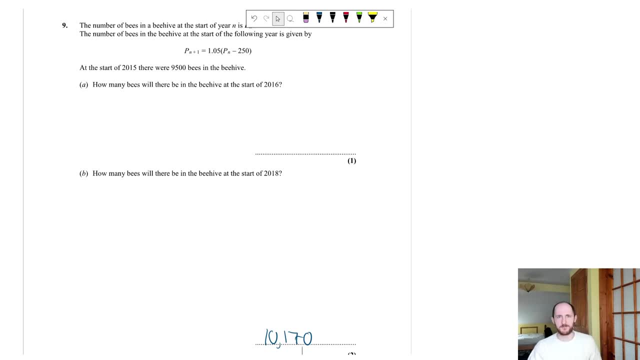 or 0.906 of a bee. this question is also pretty tricky. you have this coordinate geometry, we have a triangle here and the question is: how many bees do you have in 2017 and how many bees do you have in 2018? so the question originally just said: find an equation for the line that passes through c. 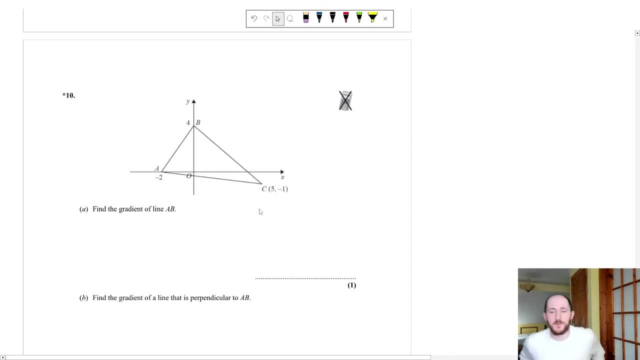 and is perpendicular to ab, and a lot of students got confused. so again, here are the steps that I would take. I would find the gradient of ab. how to do that? well, it's difference in y over difference in x. so in this case the y value is 4, here it's 0, so it's 4 minus 0 over. well, this x coordinate is 0.